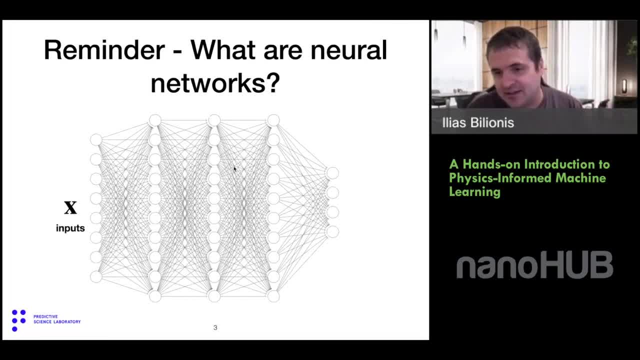 It basically looks like this: It takes some x's, which we're going to call inputs, and it produces some outputs, And basically all these links that you see represent a transformation from x to y, a function from x to y, And this function is basically a. 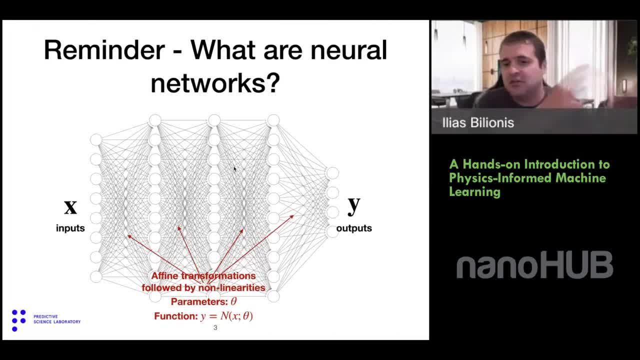 series of affine transformations, which is linear transformations, plus some biases parameterized by some weights and biases which are going to collectively call theta. So the whole thing is basically a function with some parameters, theta- okay, And I'm going to use this notation right here. 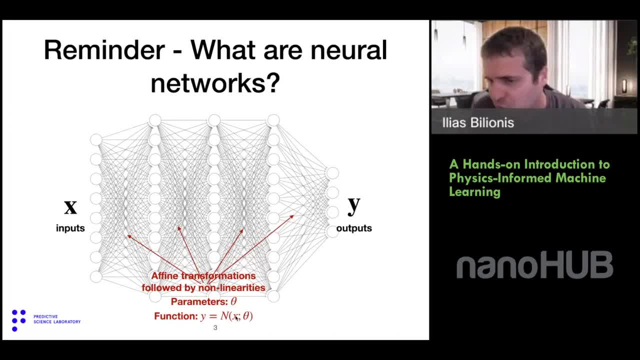 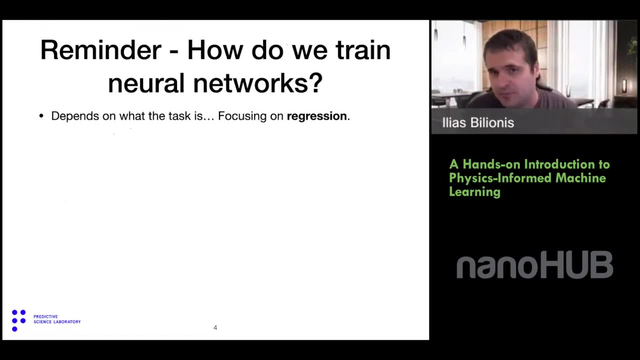 which you can read: N is a neural network that takes the input x, has some parameters- theta- and produces an output- y. okay, So that's what a neural network is. Now, how do we typically train neural networks? Well, it depends on what you want to do with that. So, if you're doing supervised learning, 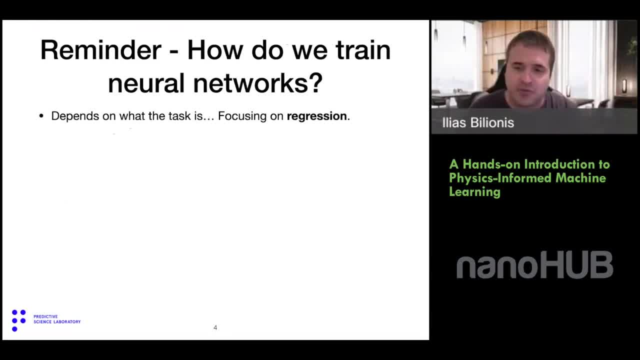 like regression or classification. you do certain things. If you're doing unsupervised learning, like the reduction function, for example, learning how to do density estimation, you do a different thing. I'm going to tell you a little bit about regression because I want to remind you of 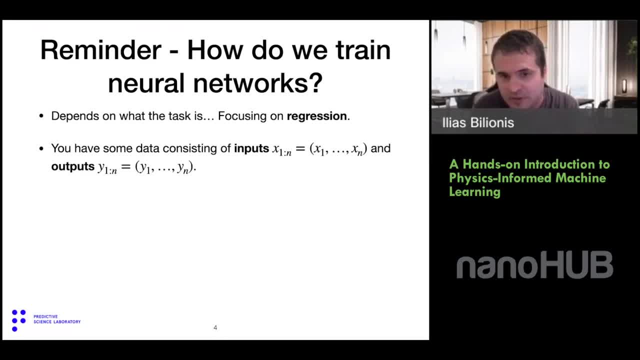 the classical things you do when you train your networks, which is you're minimizing the loss function. you're using stochastic gradient descent. So let's go over regression very briefly. In regression you have a bunch of inputs, the x's. 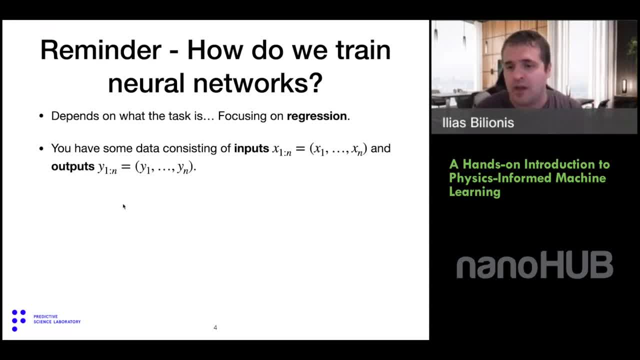 you have here, and you have a bunch of outputs, the y's, and your problem is to find the map from x to y. okay, And the way you typically do that. you want to represent this map with a neural network, of course, and the way you do it is by writing down a loss function Here. 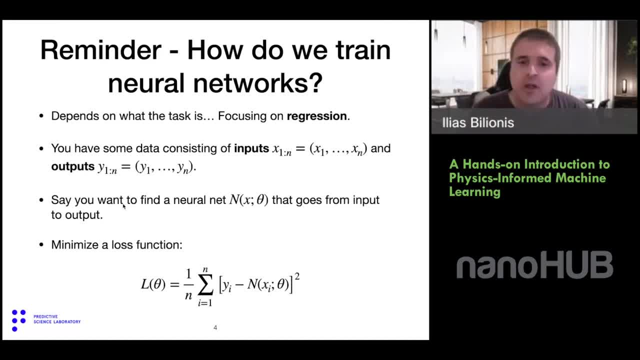 this loss function is the sum of square errors and you want to minimize it. And if you have enough data and not too many parameters, when you minimize this you're going to get a nice fit to the map from x to y- very classic stuff, Alright. the final thing I want to remind you: 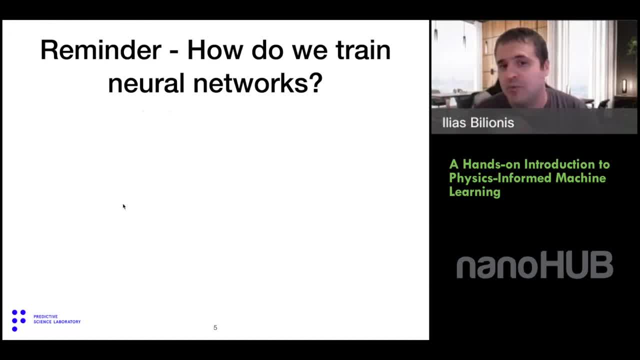 is how we actually solve the numization problem, Those we're going to use the same algorithm to play with physics and following neural networks, And what we do is we follow what is known as stochastic gradient descent. So it looks like this: So you update the parameters. 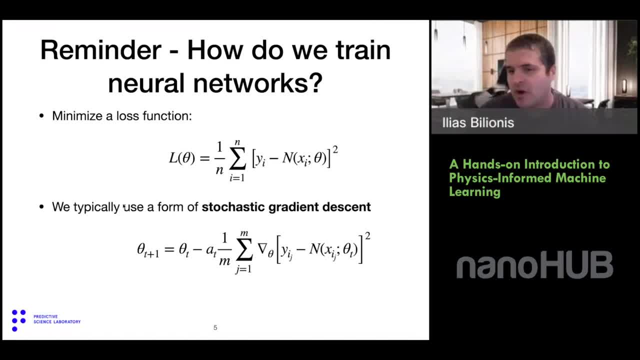 iterating, You start from some arbitrary, random, the selected parameters, and you change them a little bit and you change them in the opposite direction of the gradient of the loss. But the gradient of the loss, typically, because you have lots of data, you estimate it through. 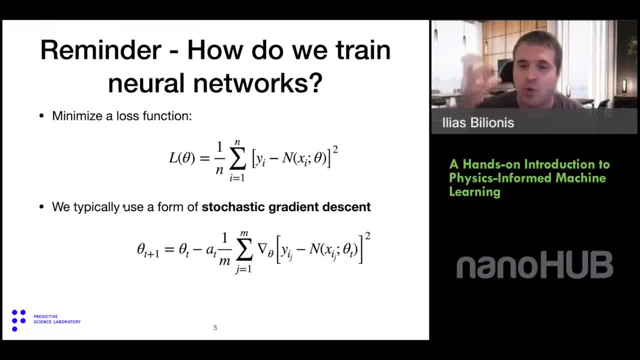 what is known as the sampling average approximation. that's where the stochastic part is coming from. So these Xs and the Ys- and not all your Xs and your Ys, but a randomly sampled subset of these- is called the BATS. 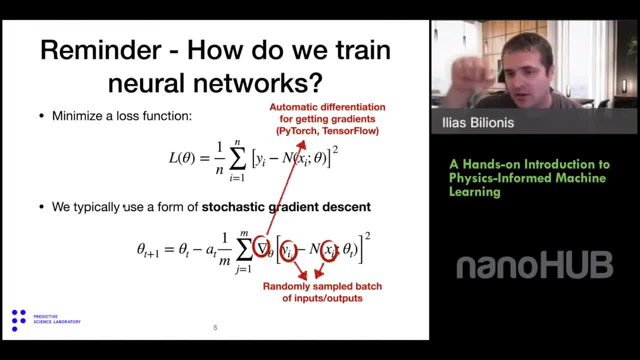 And these gradients of the loss with respect to the parameters of the neural network. Theta is coming automatically through a package like PyTorch or Terms of Load, so we're using automatic differentiation to take these derivatives without actually coding this, And we're going to use PyTorch today to take derivatives whenever we need them. 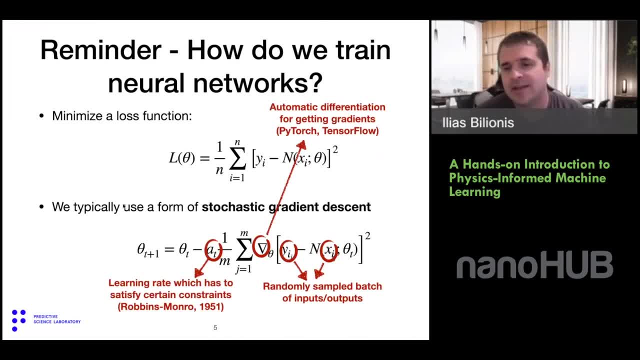 And this term right here is called the learning rate, And this term right here is called the learning rate, And this term right here is called the learning rate. And it has to satisfy certain constraints so that the algorithm actually converges to a local minimum of the loss. 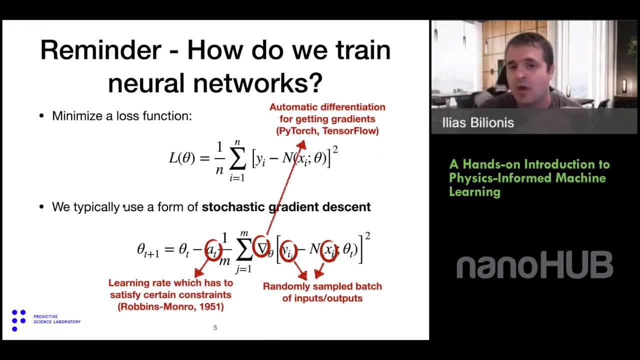 The details for that is in the Robbins Monroe 1951, a very, very famous paper on how to select these learning rates. that first would prove that this algorithm converges. It's important to remember that when we are setting this up, we need to know what are. 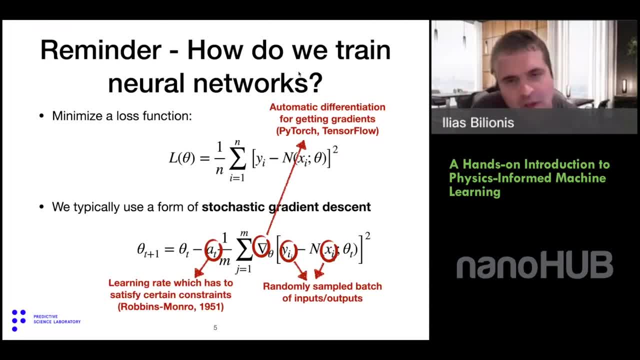 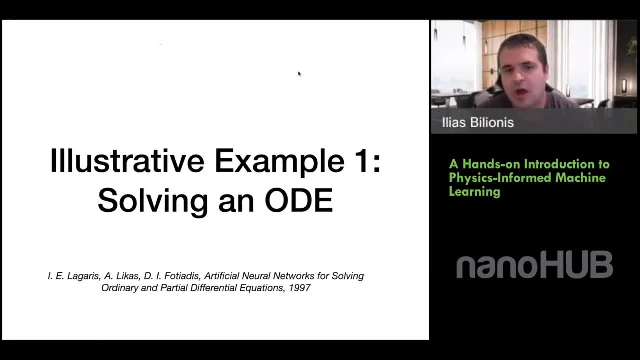 the requirements for convergence, Otherwise it may never converge. All right, so I'm going to start with an illustrative example. I'm going to show you how you can use neural networks and loss functions to solve an ordinary difference equation. And notice that this paper is written in 1997, so it's 24 years old. 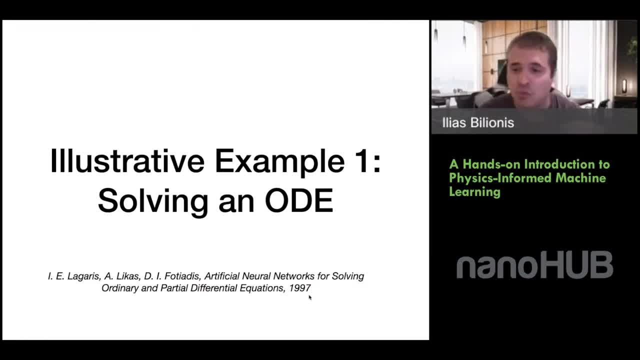 It's quite, quite old, okay, It was completely ignored for basically two years. It was completely ignored for basically 20 years- like no citations whatsoever for 20 years. And then, all of a sudden, the whole thing got revived and the paper probably has right. 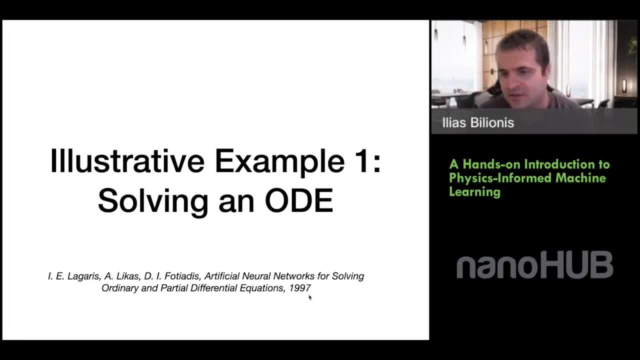 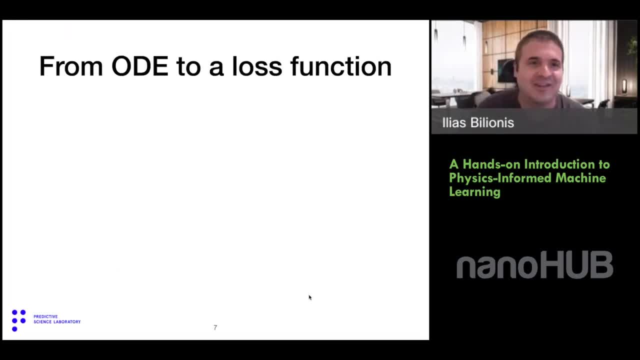 now thousands of citations, all within the last two years. all right, So this is something to remember. your work may be recognized a lot later. All right, so this is, let's do it. let me show you how you can use neural networks to 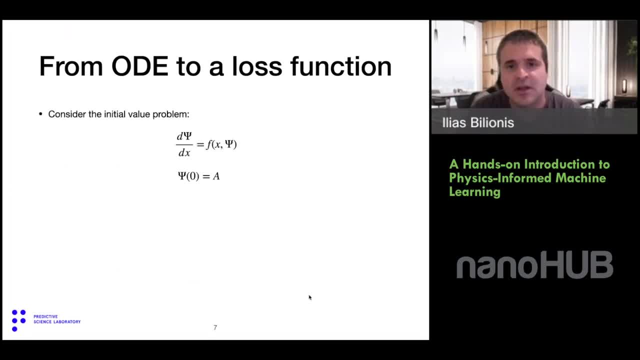 solve all these ordinary difference equations. Here's an ordinary difference equation: the derivative of psi is equal to something and you have some of these conditions. psi zero is equal to A. So the first thing we're going to do is we're going to parameterize the solution: psi, essentially. 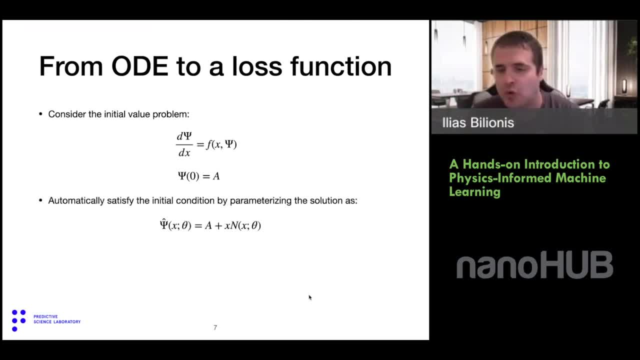 using a neural network. Now we're going to be a little bit smart about it. We're not going to make psi a neural network. we're going to parameterize psi in a way that automatically makes it a neural network. We're going to make psi a neural network. we're going to parameterize psi in a way that 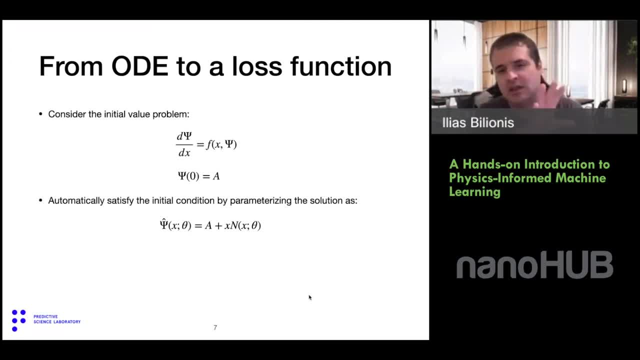 automatically satisfies the initial conditions. This is a very common trick in numerical solutions or differential equations, either ordinary or partial. You basically it's a special form. If you plug in x equal to zero, you basically get the initial condition, okay. 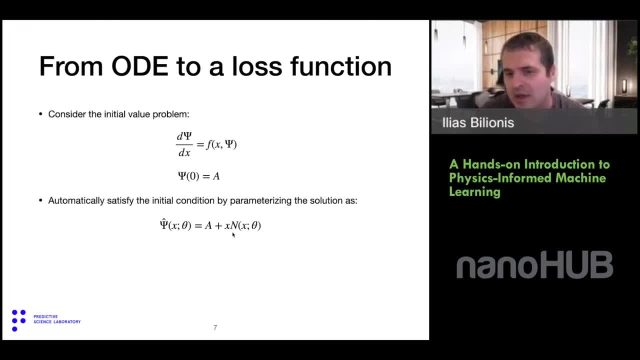 That's the trick. Now, this term right here is a neural network which has parameters theta, and we have to find the parameters theta so that this equation, the partial equation, is a neural network, The partial differential equation, the ordinary differential equation, is satisfied everywhere. 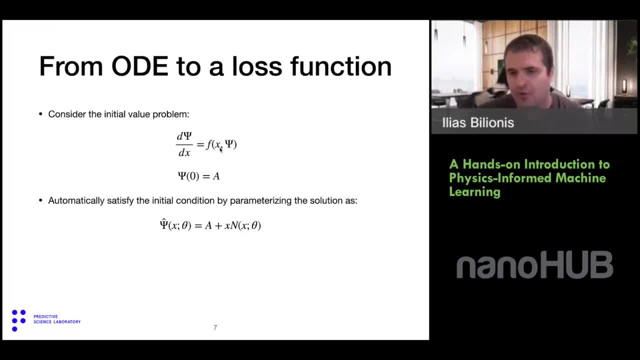 for all x's, Of course, from x equals zero up to a big number, And we don't have to worry about the initial conditions. because of this trick, they're automatically satisfied. Here's the idea. Here's the idea presented in that paper by Lagares in 1997.. 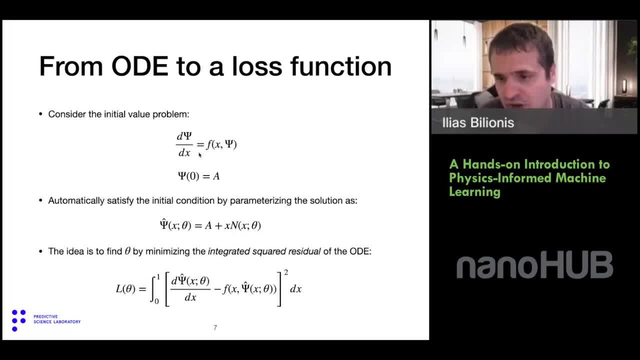 You take you need to make a loss function to train a neural network. okay, So how do you make that loss function So that minimizing the loss function is equivalent to solving the partial differential equation, the ordinary differential equation. So here's how you do it. 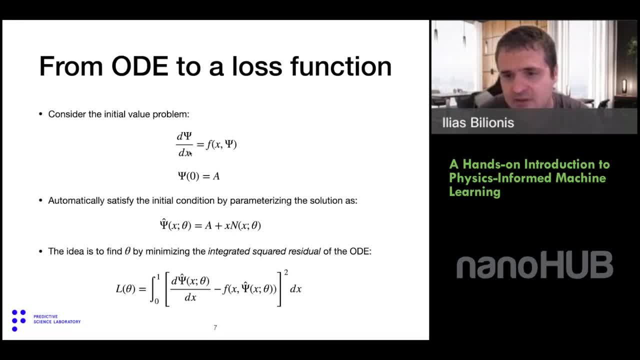 You take the differential equation, you move everything to one side, you square it, so you create the square residual of the differential equation, and then you integrate this thing over all the x's, Of course. here we go from zero to one. 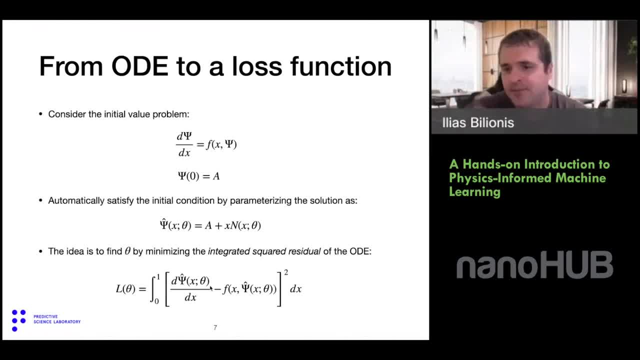 So now, if you minimize the loss function, you get the differential equation. You take the differential equation, you move everything to one side, you square it, so you create the partial differential equation. If you minimize this exactly, so if you bring it down to zero, basically you have found: 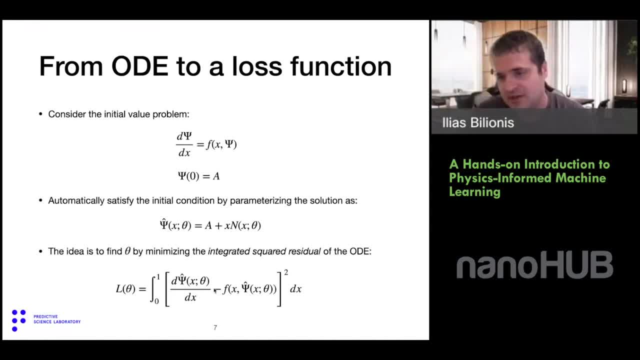 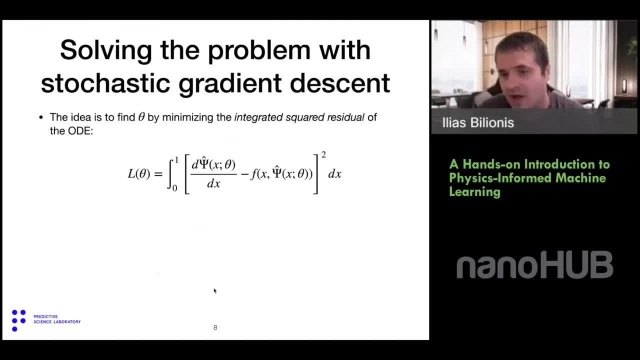 a neural network that solves the ordinary differential equation. That's the idea. All right, How do you solve this problem? Let's say you have an integral right. You don't have a finite amount of data, So the integral is essentially equivalent to infinite x's. 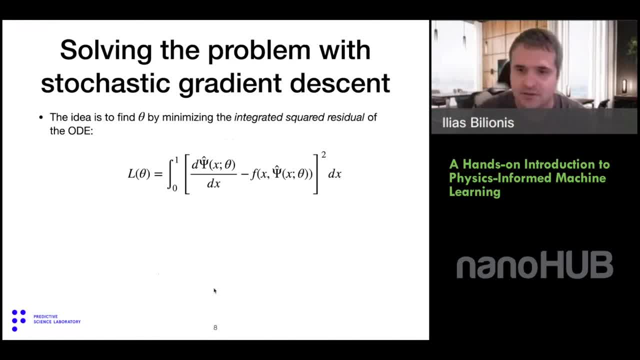 That's what it is equivalent. It's the summation of all the x's Continuous summation. Okay, So you can still use the idea of batching. There are some details here to show that this algorithm- stochastic gradient descent- written down like this, actually converges to the local minimum of the loss function. 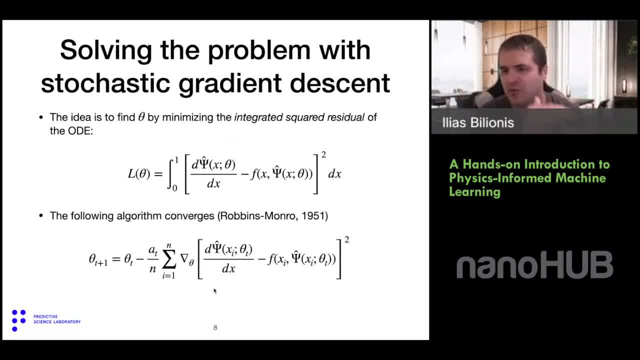 We're going to skip these steps. It's pretty straightforward. If you're interested in it, you can take my class. I talk about it there, But this is the algorithm that we would use to minimize the loss function. Okay, So you can minimize the loss function of both. 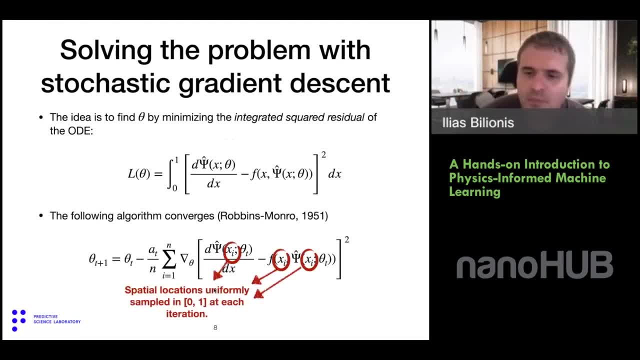 Look at this, These x's right here, they're randomly sampled points, randomly sampled x's between zero and one, uniformly sampled, And you can see that if you do it this way and the learning rate is just right, this will converge. 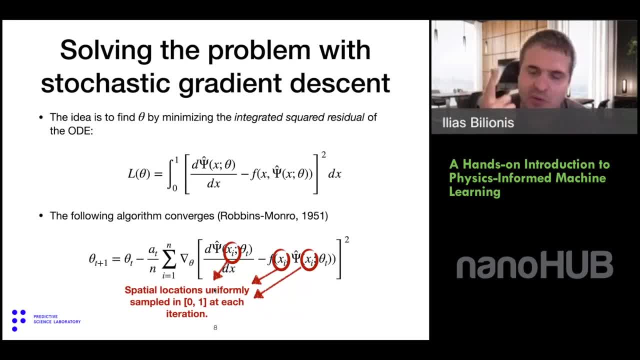 And it will converge even if you just take one sample per iteration. So you just pick one x per iteration, it will still converge. Of course, the more samples you take per iteration, the less variance of the algorithm, the more it will converge. 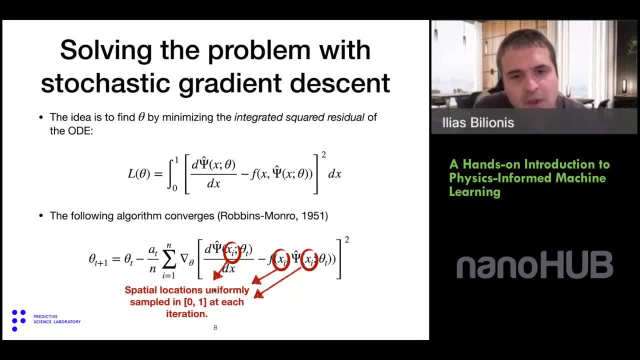 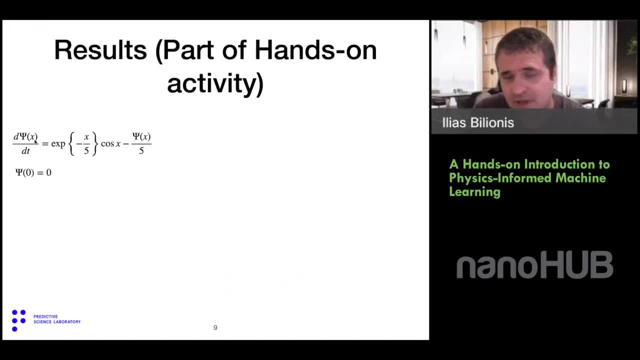 And the faster it will converge in terms of iterations. Okay, So that's pretty much it. So, in the hands-on activity, the very first thing we're going to start with is solve this really trivial differential equation, which I have an exact solution. 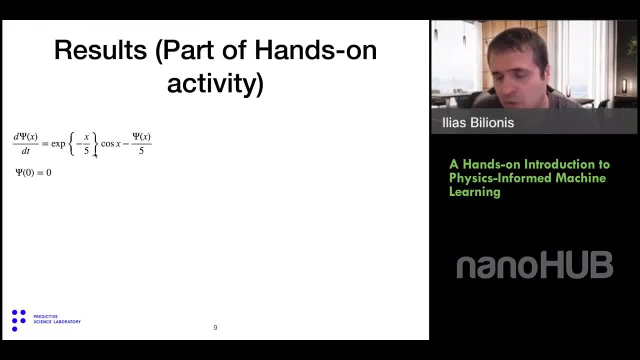 So you can compare that doing this thing with neural networks will actually recover the exact solution. So you're going to do this hands-on activity after I'm done. This is the kind of plot you're going to see. You're going to see basically a perfect match between the two. 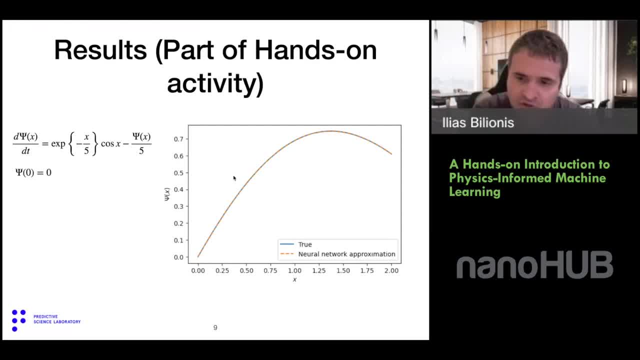 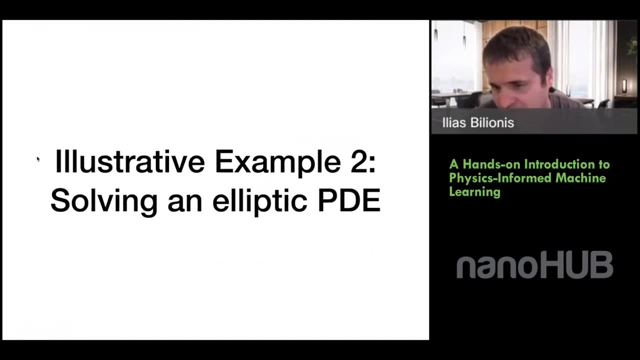 Okay, You're going to see a perfect match between the true solution to this initial value problem and your approximation with neural networks. Okay, All right. Illustrated example number two: let's use the same idea to solve partial differential equations. You'd be surprised. 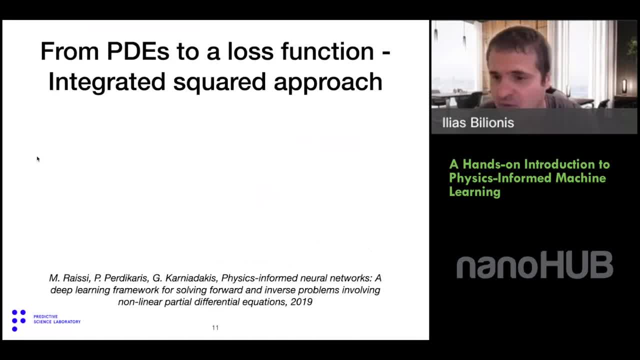 There's actually nothing new here. It's the same thing we did before, only with partial differential equations. Here's a standard elliptic partial differential equation. It appears everywhere, from magnetostatics to elasticity, to heat transfer, flow through post-media ubiquitous equation. 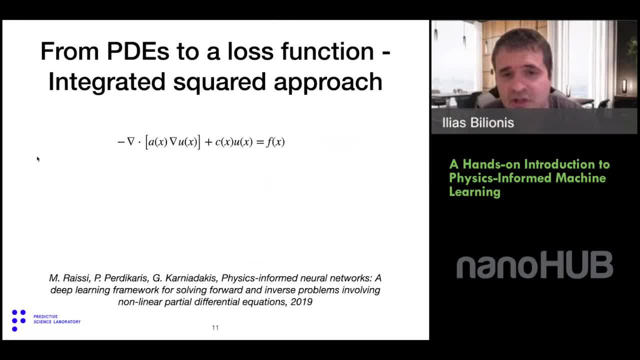 And we want to solve this with neural networks. so we're going to parameterize U so that it satisfies some various boundary conditions. let's say: What you do is you take the left-hand side, you move it to the right-hand side, you square. 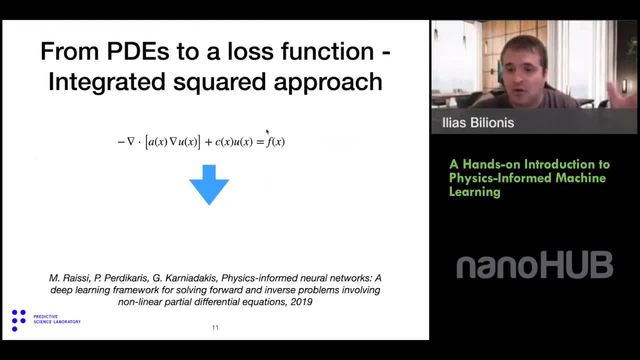 the residual and you integrate over space. Okay Now, X is not necessarily one-dimensional, It could be two-dimensional or three-dimensional. Okay, So that's how you make a loss function, the minimization of which is equivalent to solving the PDE. 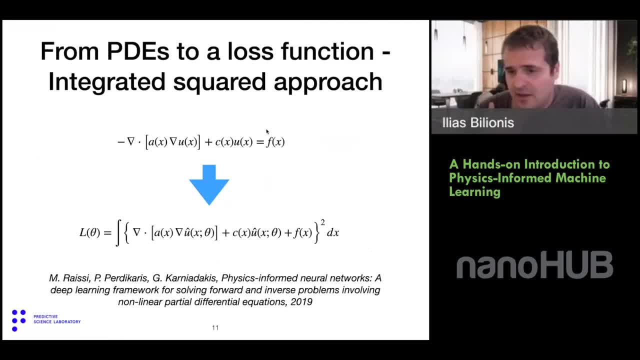 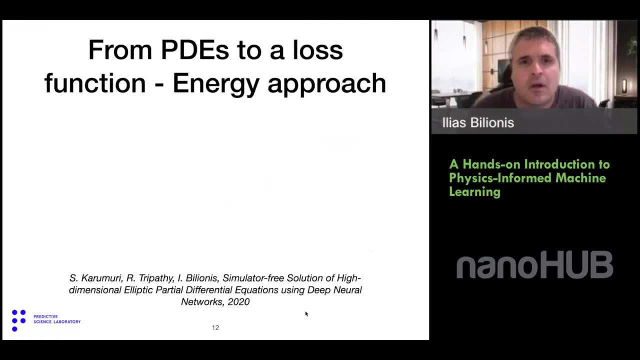 Okay, And that's the idea that revived Lagari's paper, And the first new instance of this is on this paper. All right, Now, using the integrated square residual, so moving everything to one side. squaring integrating is one way to do it. 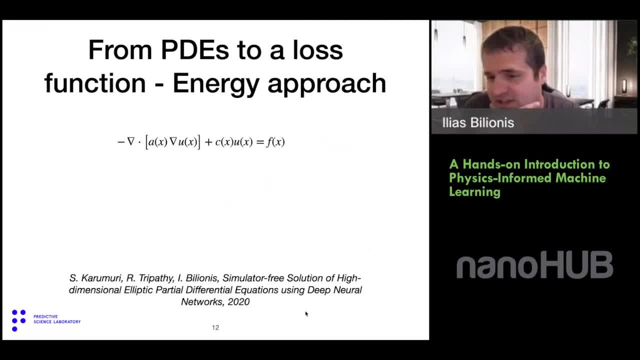 We have shown in our own work that it's not necessarily the best way to do it, because the loss function doesn't necessarily have a solution. Okay, And in some physical problems, in this part of the physical problem in particular, which is analytic PDE, there's a mathematical theorem called the Dirichlet principle that shows: 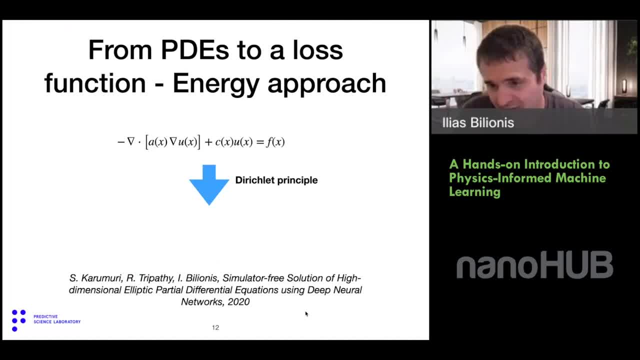 you that solving this PDE is equivalent to minimizing this loss function, which is essentially the energy contained in the U field, And so the mathematical proof says that this loss function is equivalent to the loss function. Okay, So minimizing this loss function, the energy functional- has a unique solution and the 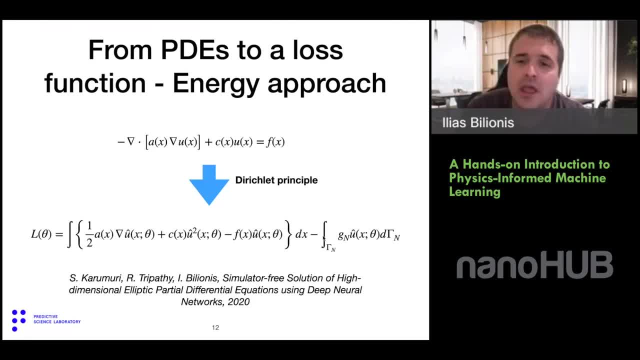 solution satisfies the PDE And you see that it's different than the integrated square residual And it also has this term right here, which is the natural boundary conditions, which didn't even appear in the other formulation. You have to introduce them by hand. 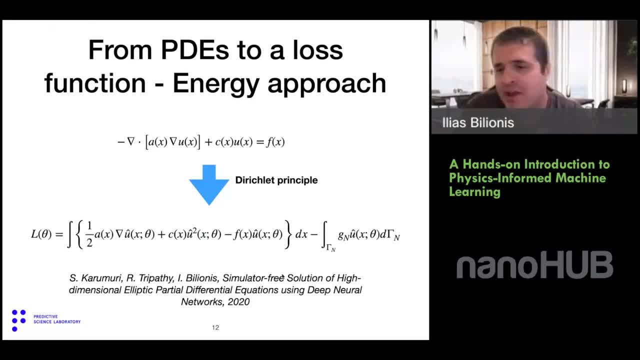 So take-home message: whenever there is an energy formulation for your ODE or PDE that's actually better to use than using the integrated square residual, because it usually has a unique solution. It behaves better in general, All right. Why is this useful? 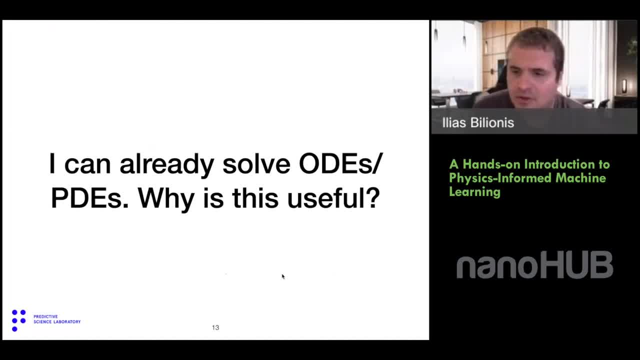 Why should you care? You already know how to solve ODE and PDEs, So, on that regard, this is completely useless. Okay, So let me tell you why it's useful and why you should pay attention to it. The reason is not that you can solve a single ODE or a single PDE. 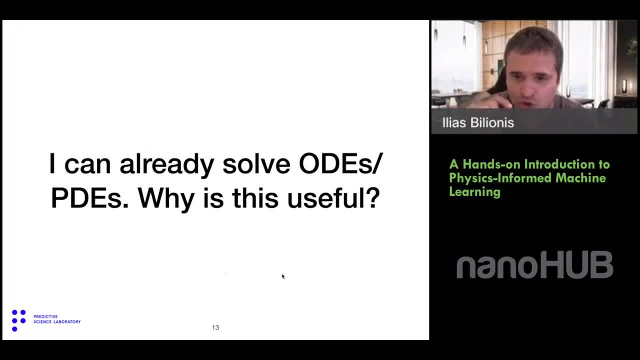 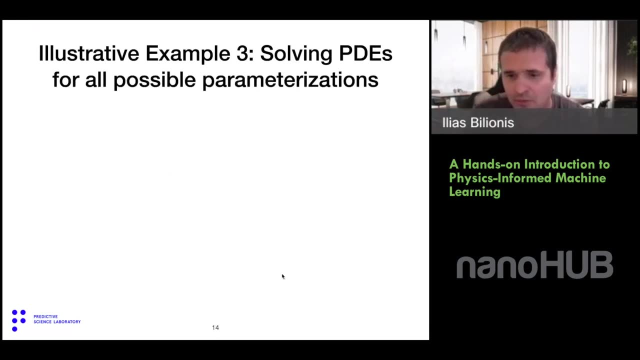 The reason is because you can generalize this technique to solve PDEs for all possible parameters, for all initial conditions, for all boundary conditions in one sweep. Let me demonstrate this Through an example from ROP. So here's a PDE, just like we had before, an elliptic PDE. 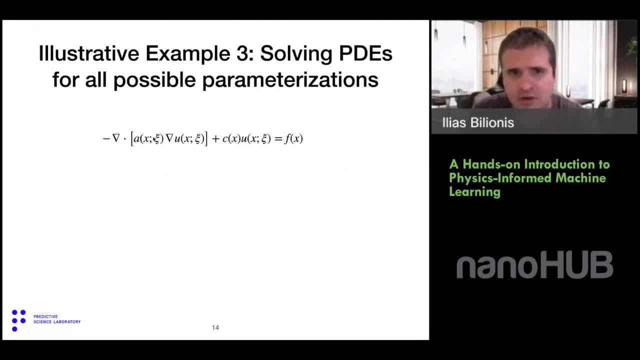 Only now notice this term: A here, which you can think of as a thermal conductivity, for example, of a material, is parameterized by xi And you can think of it as random And you want to solve. there's not a single PDE here, there's a PDE for each realization. 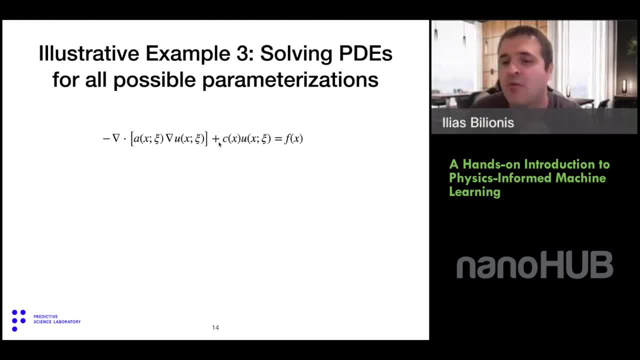 of xi And you want to solve this PDE for all the xi's at once. Now let me give some boundary conditions Also, I'm going to operate on a box. We have these basic boundary conditions, natural boundary conditions like that. xi are the random parameters. 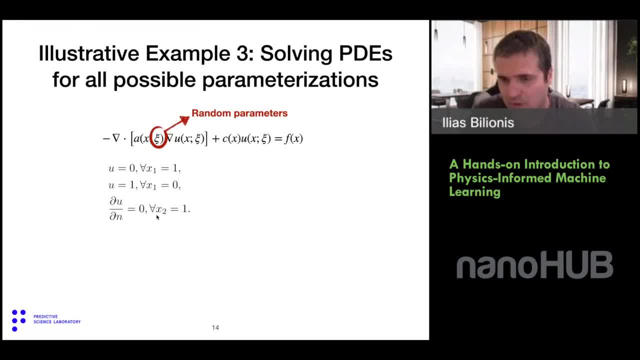 We want to solve this boundary value problem for all xi's And I'll tell you how the The the log of the conductivity would look like. So it could look like this. So it's basically a picture And it cannot be described with one or two parameters. 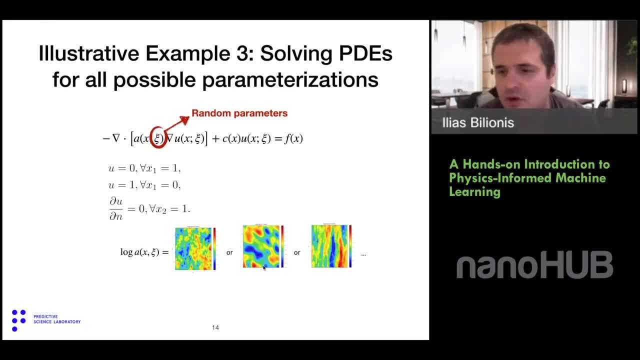 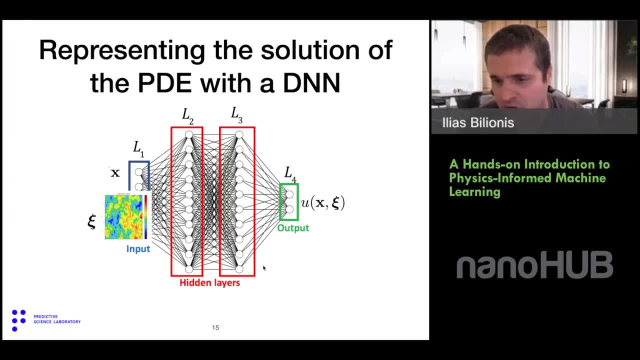 As a matter of fact, it requires a few thousand parameters to describe this picture And we want to solve the PDE for all such pictures. So we want to be able to plug in such a picture, give a neural network a picture and give it a special location. 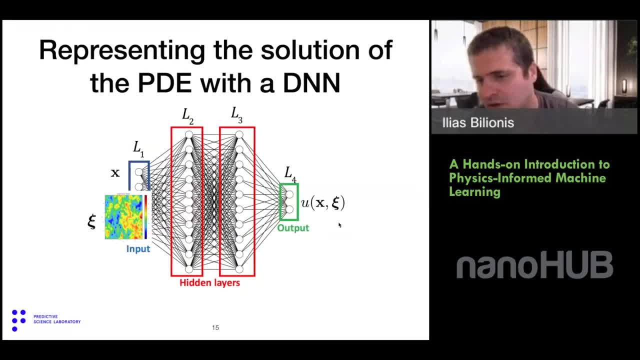 And it's going to tell us what is the temperature of that location, if that was our conductivity, And that you should satisfy, of course, the PDE that we showed you before for all oxide. That's the problem we want to solve. 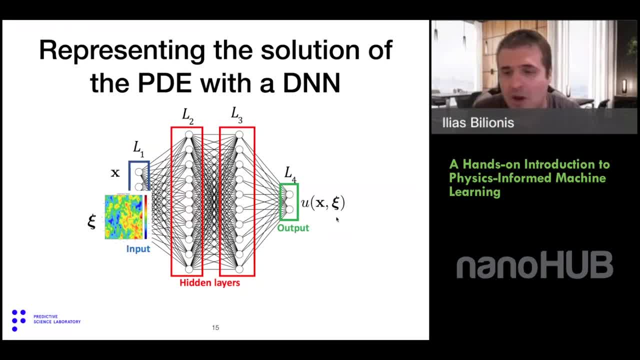 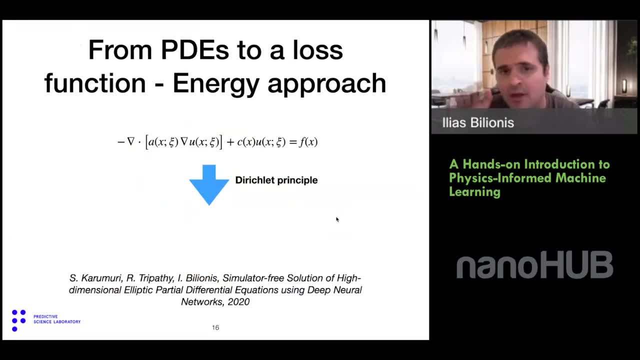 And that size is basically described by about 1,000 pixels in this particular example. So how do you do that? You use again the Dirichlet principle, but in an extended way, To get this loss function. So notice that what we have inside 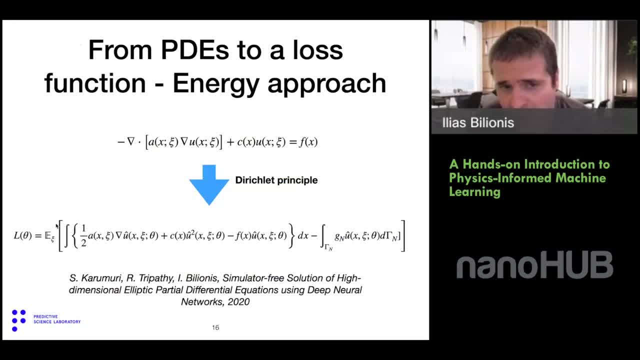 is the loss function we had before, But now we have included an integral over all the parameters. So what do you do? You basically treat the parameters just like you treat the spatial variables. You integrate over them And that gives you the loss function. 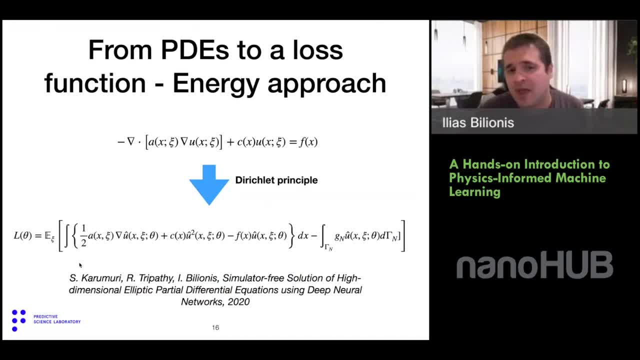 And for this particular loss function we prove in this paper that if you minimize it then you can get a mixed solution. If you minimize it, you're solving the PDE for all oxide, All right. So if you do stochastic gradient descent for a neural network. 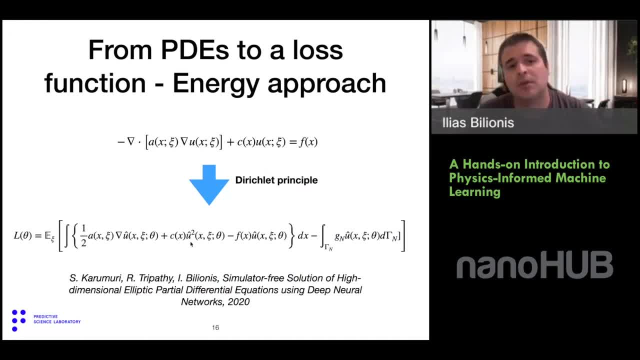 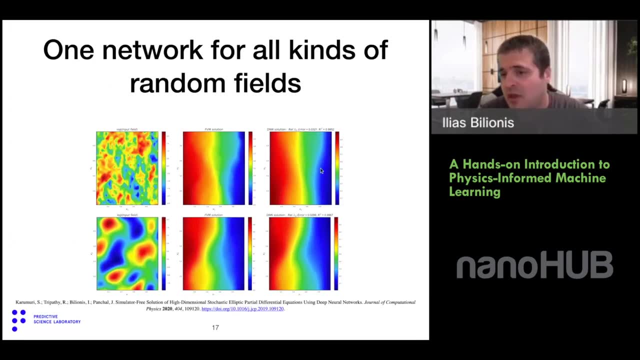 that represents the solution here. it will convert to the solution of the stochastic price of the. It will solve this for all oxide And then you're going to be able to feed it whatever picture you like, And it's going to respond with a prediction. 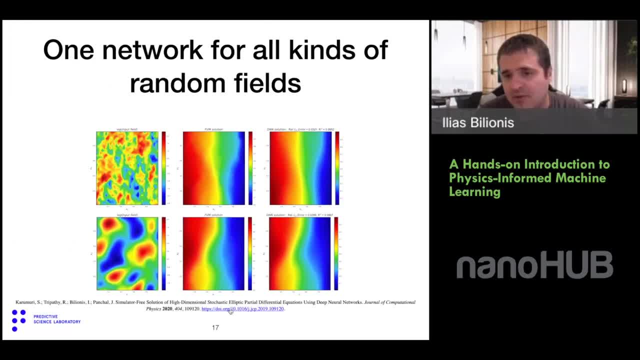 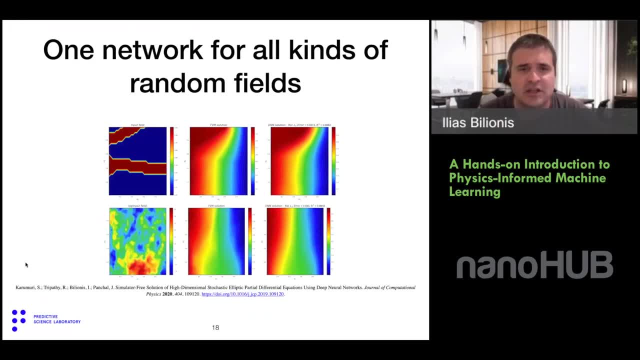 Here you see the Solution with five volumes for this particular oxide And here you see the prediction of the network And you can see that you can feed it basically whatever you want, And it will still provide quite good results. Now, back then when we wrote this paper, 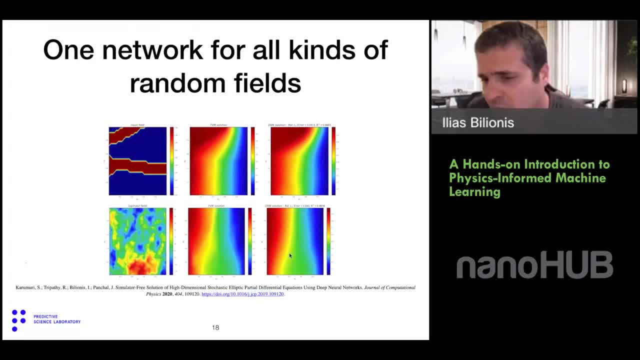 if you notice carefully, you will see that the neural network is missing some of the fine features of the solution. Back then, when we wrote this paper, we didn't know about how to make this better. There is an issue with neural networks in general. 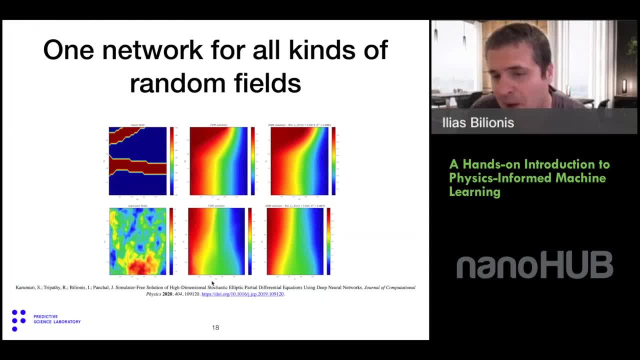 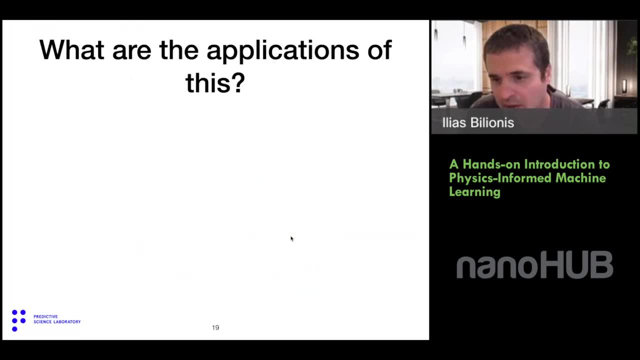 known as the spectral bias, which came up around the time we published the paper. Now that we know about the spectral bias, we can actually make OK. So what are the other applications of all this? Just to give you a. So we talked about high-dependence. 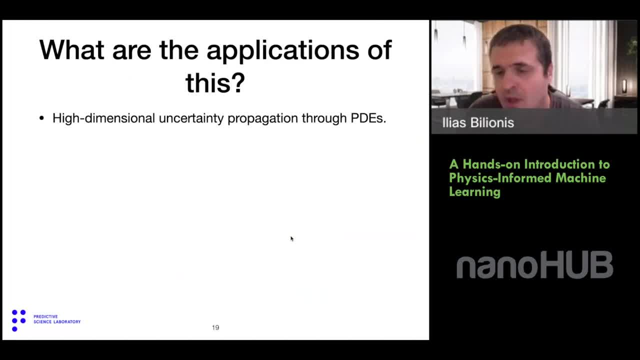 on propagation through PDEs. That's one application And you can imagine that this is just one PDE. You can go and do it through equation, You can go and do it through the elasticity equation, You can go and do it through the Schrodinger equation. 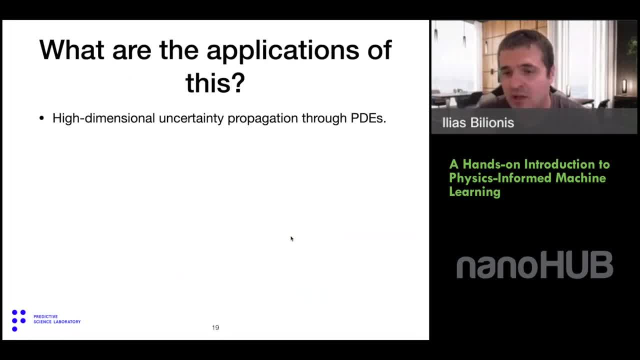 You can go and do it through the And as soon as you have a PDE with parameters, you can use this technique to solve the PDE for a parameter. You can solve, use, you can formulate and solve ill-defined PDE problems. 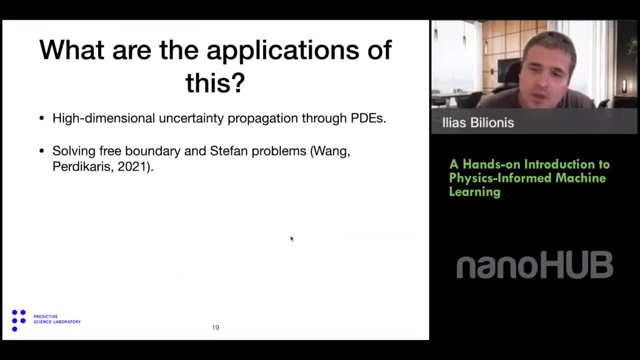 like problems with three boundary problems. You can see paper on that. You can do PDE constraint optimization. So there is a paper- recent paper- by NVIDIA- It's not previewed yet but you can find it and read about it- where they basically design a heat sink using this idea. 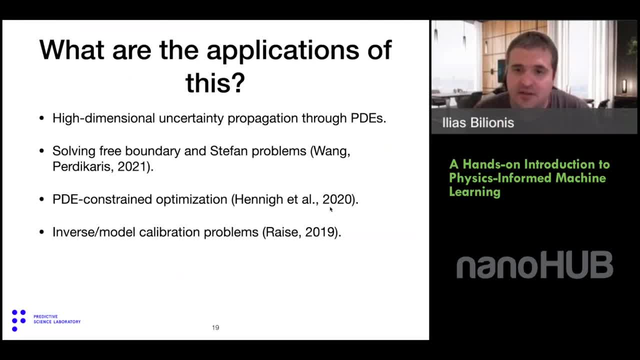 And, as a matter of fact, last year there's a video presented in his keynote speak this particular work. You can use the idea to do all the calibration. So you have a PDE with parameters And you want to identify the parameters using some data. 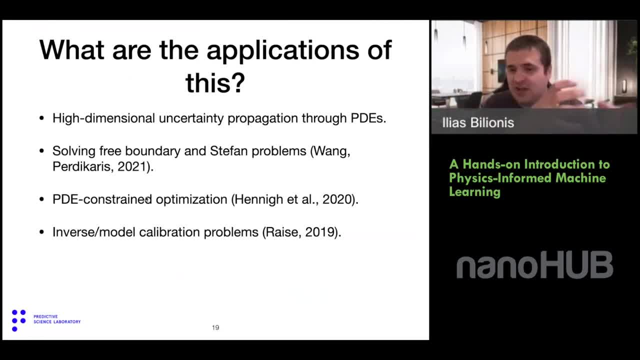 And you can make a loss function, one part of which has your data. The other part has the physics-based part of the loss function. You weight the two things And you minimize the weight of some of them, And this could solve the problem. 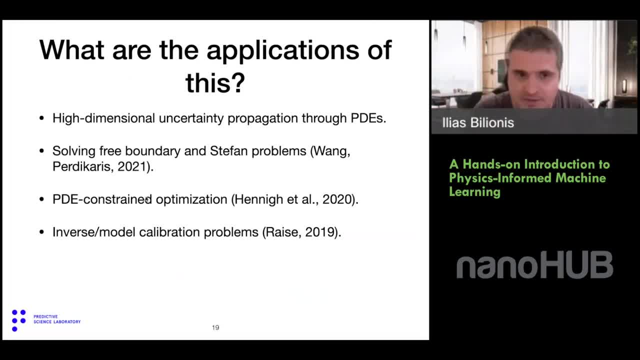 Of course it will have to be a well-defined problem And you could use this idea to do data simulation And we have a time-dependent measurement And the underlying field satisfies some time-evolving PDEs. You could use data to reconstruct the underlying fields. 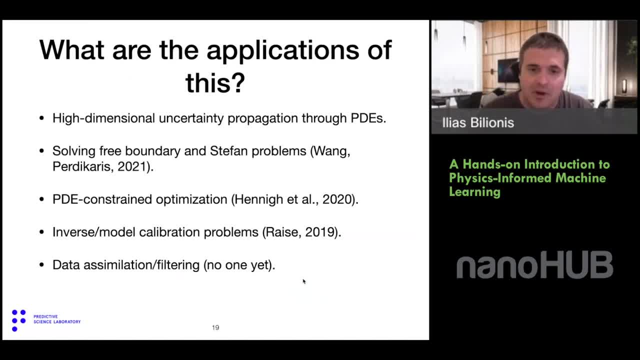 So these are some. We're working on this with Particle, As a matter of fact, is also has a paper on this that came out a while ago, And I will go as far as say that at least my community is going to be engaged in this for the next four or five. 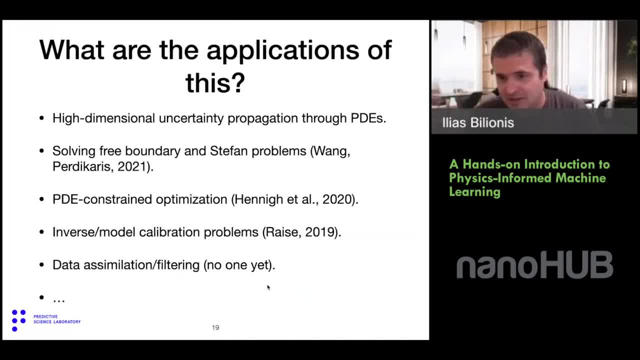 years. As a matter of fact, we don't have yet a next big thing. This is our next big thing. It could be the solution to our problems, Because it's really straightforward to formulate the problem: You just need a loss function that we can make out. 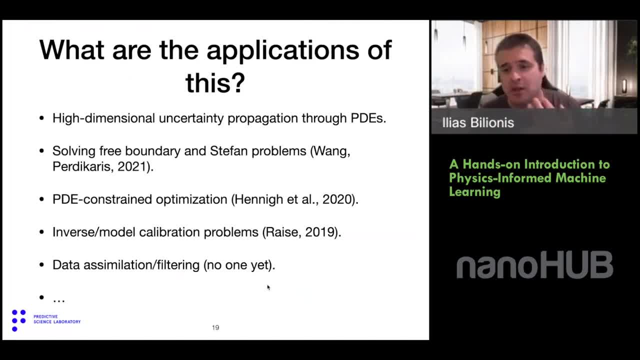 of the physics, And then you just request a super simple. The neural networks scale very well with increasing dimensions, And all our methods for answers- qualification, for example- suffer from the curse of dimensionality. Deep neural networks suffer less, So I think we're going to be seeing more and more of this. 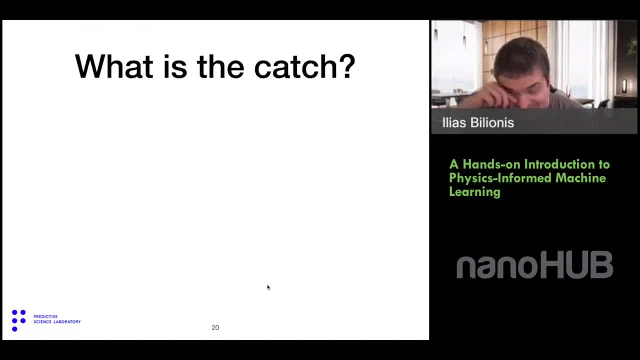 in the near future. All right, so what is the catch? The catch is that if you try to apply it to your problem, it's not going to work, And unless your problem is very, very, very simple, it's not going to work. 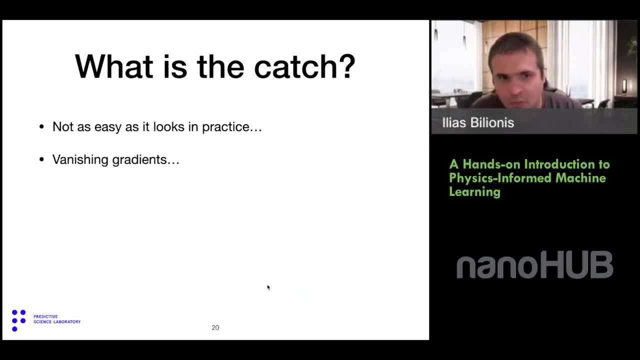 And there are many reasons why it's not going to work. There is a problem of variance in gradients. This is a common problem in neural networks, especially deep neural networks: The gradients. if you make them too deep, they are very close to zero. 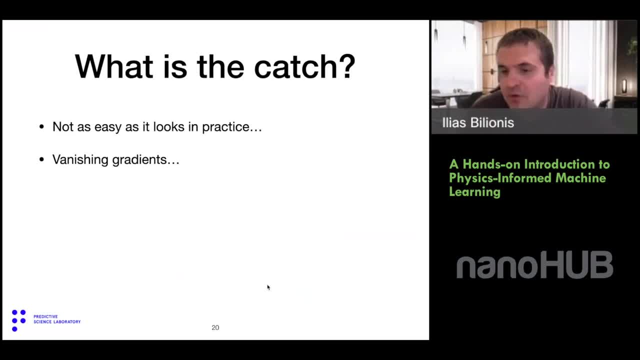 And there's the. The gradients don't move them. So theoretically it will convert, But in practice it never converges in a reasonable amount of time. There is a way to fix this. You can use residual connections. We show you how to do this in the 100 activities. 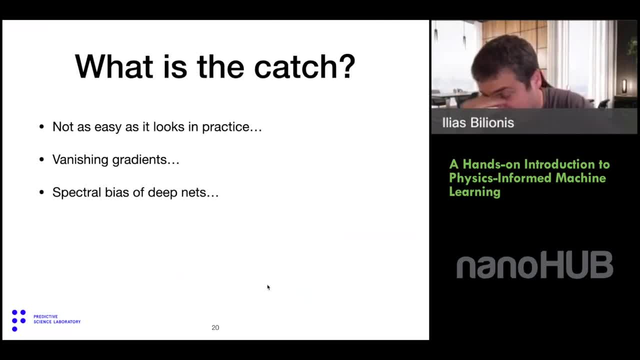 There's a spectral bias of deep neural networks, which is something that we discovered theoretically, basically last summer, And the spectral bias can be described as follows: And neural network first learns low frequencies, It learns small things And it will eventually learn the high frequency. 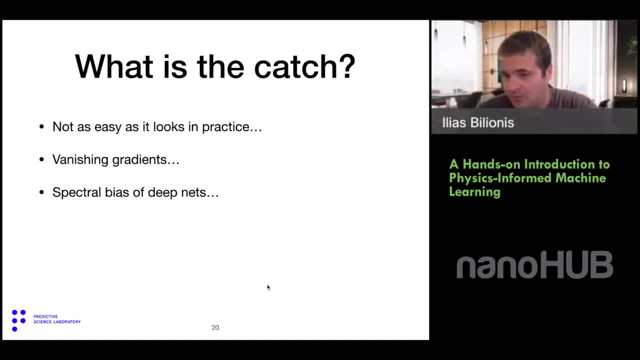 content of a function, But it will take forever. So if you are solving a PDE, for example, that has a SARP featuring solution, it will find, let's say, the mean, And then it will take forever to converge to the fine details. 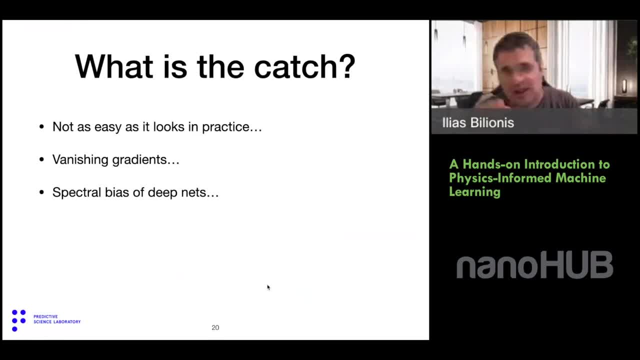 It will converge to the fine details, but it will take forever. And that's coming from the spectral bias. It's theoretically explained why this happens And there is a way to overcome the spectral bias using some so-called 3DF features at the very beginning. 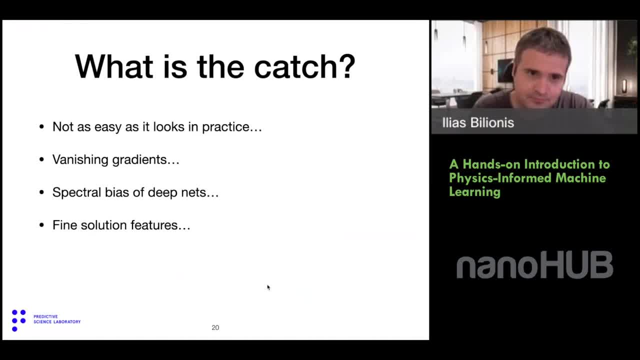 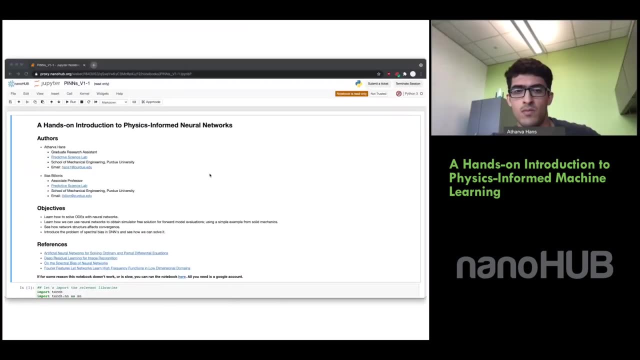 of the network And we'll show you how to do that in the 100 activities. Yes, And that's all I have. All right, So I thought about, you can take it away from here, OK. So this hands-on activity has two main examples. 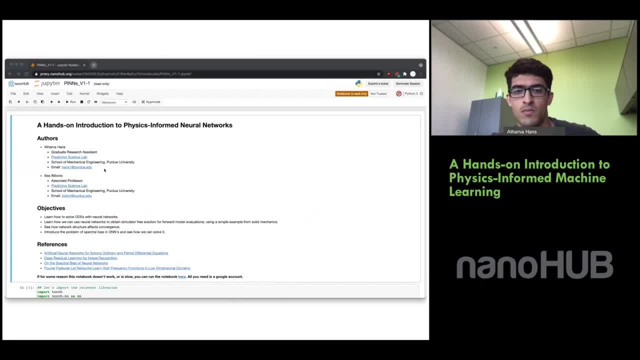 What I'll do is I'll present an overview of what we are trying to do in these examples And then maybe everyone can run the code and see how we implement these examples in PyTorch and what are the kind of results that we get. 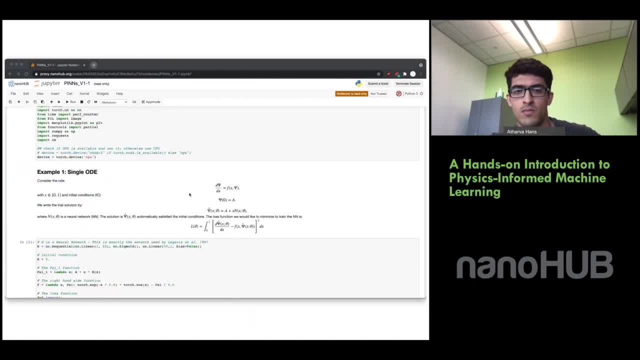 So let's begin with the first example. In the first example, we are trying to solve an ordinary differential equation using neural networks, And this is basically the same example which professor I'm going to show you. This is the same example which Professor Biljanas. 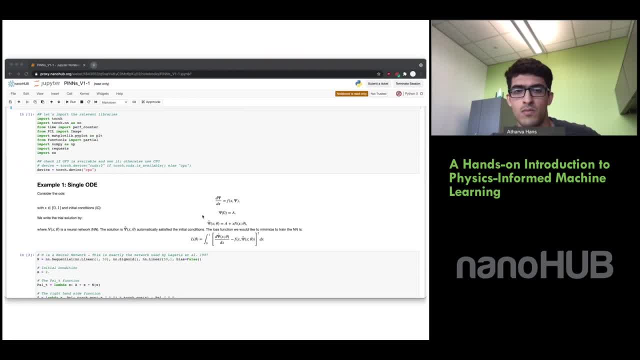 was talking about in his talk. Here, the main idea is to first represent the solution using a neural network- This is what I'm doing over here- And then the loss function that we minimize to train the network is the squared residual loss, And we obtained this from the differential equation itself. 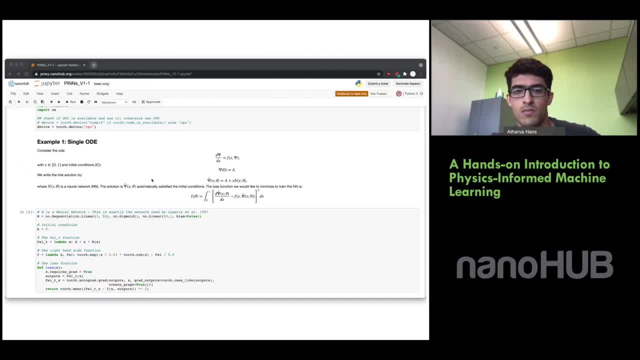 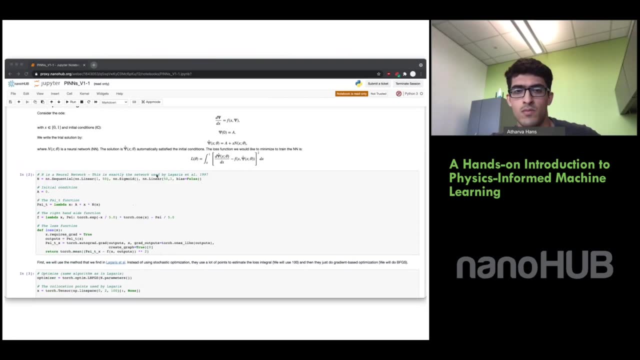 This is a pretty straightforward example And the main idea behind this example was to again show how we can parameterize this solution of the ODE using the neural network and see how we can set up the loss function. So this example kind of forms the basis of more complex problems. 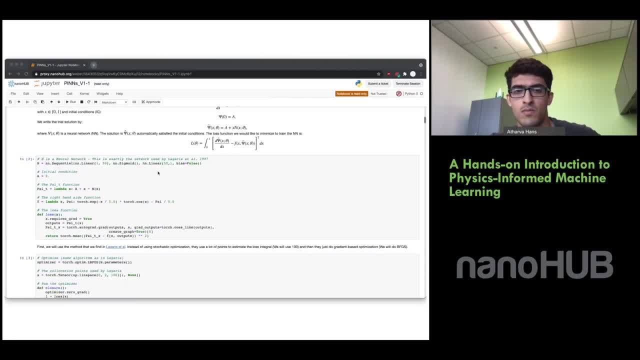 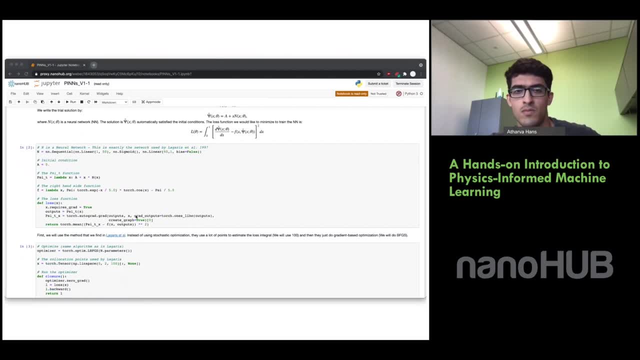 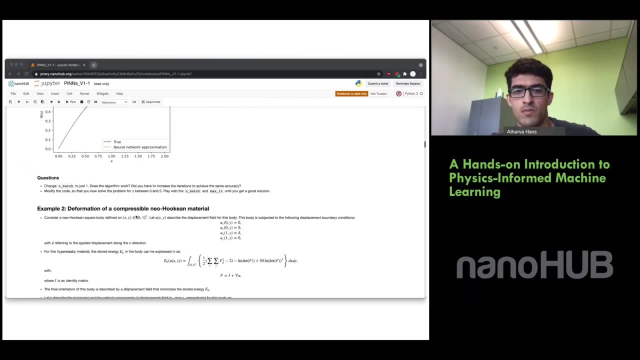 that we would like to solve using pins In the next few cells. I'm just setting up the problem And once I'm done with an overview of these two examples, you can run this and see the kind of results that we get. Moving on to the second example in this example, 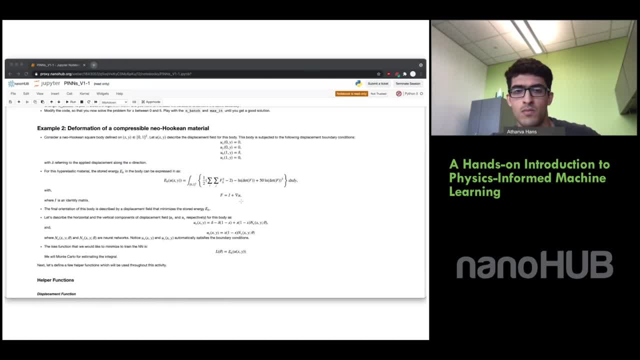 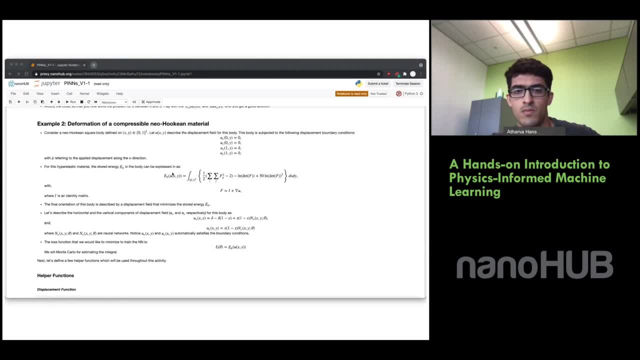 we go over how we can obtain simulator-free solution using neural networks. For this we use an example from a solid mechanics And, in particular, we have a square body which we subject to specified displacement boundary conditions, And the goal is to find the final orientation of this body. 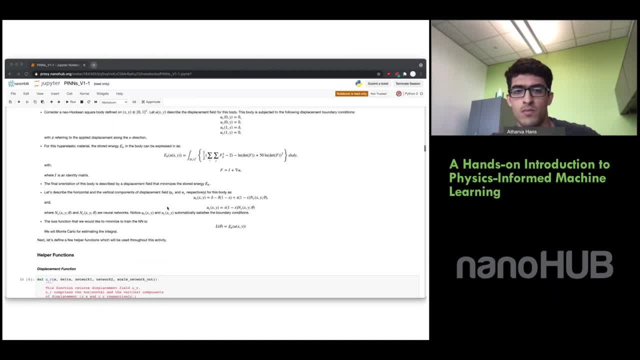 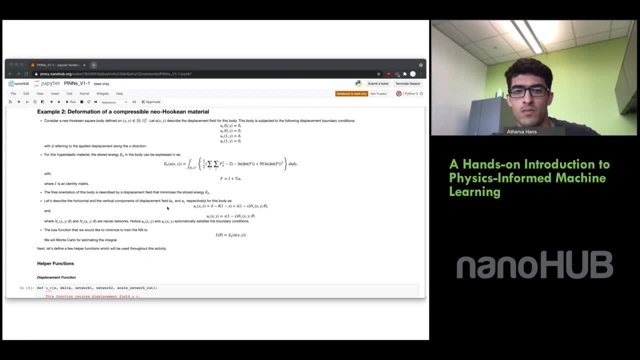 in a deformed state. Traditionally, we solve this problem using FEM. But the issue of using FEM is that it's time-consuming for large value of displacement boundary conditions, And in the notebook I go over why exactly that's the case. 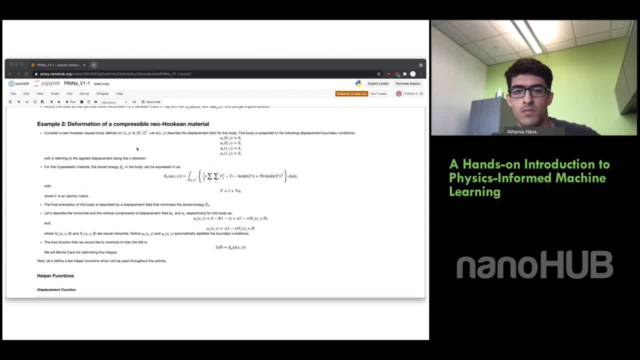 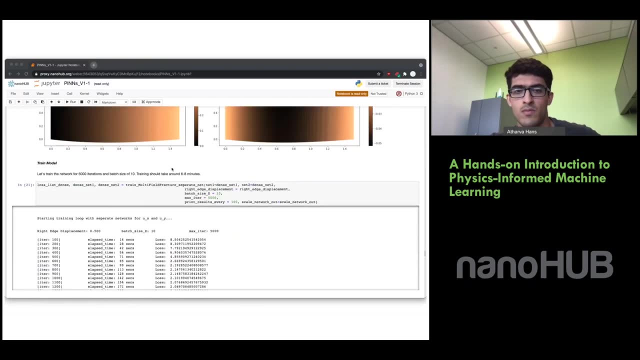 So overall, in this example I show how we can solve this problem using pins And I also go over how different network structures affect the results. So that's kind of like an overview of what these two examples talk about. Now maybe everyone can run this notebook at their end. 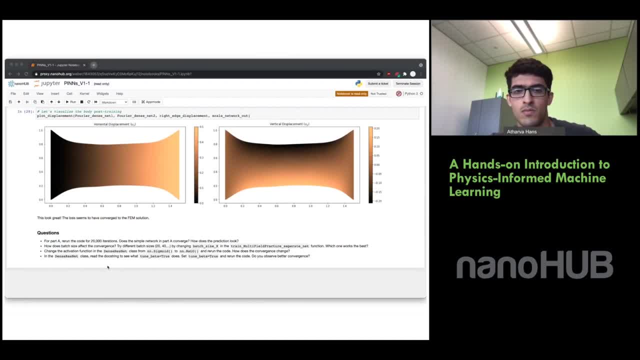 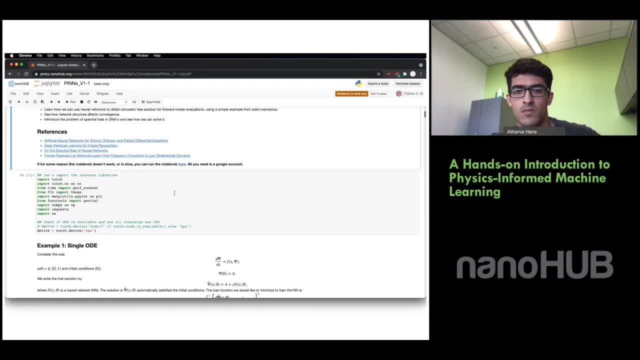 and see the kind of results that we obtain. And as everyone goes through the activity, Professor Biljanes and I can answer any questions that you might have. So in the first cell I'm just importing the relevant libraries And in the second cell I'm first defining a function. 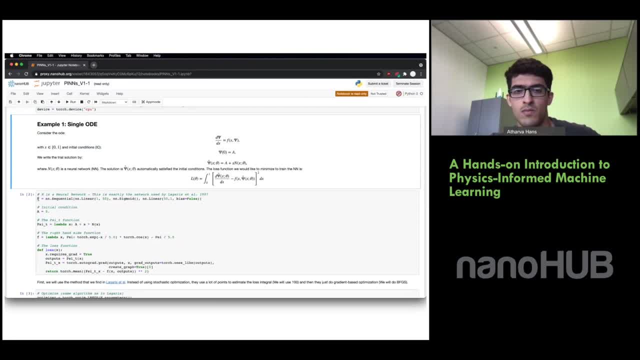 And I'm just going to import the relevant libraries. And in the second cell I'm first defining a function, And in the second cell I'm first defining a function. And this is the kind of look like we've done in our network. 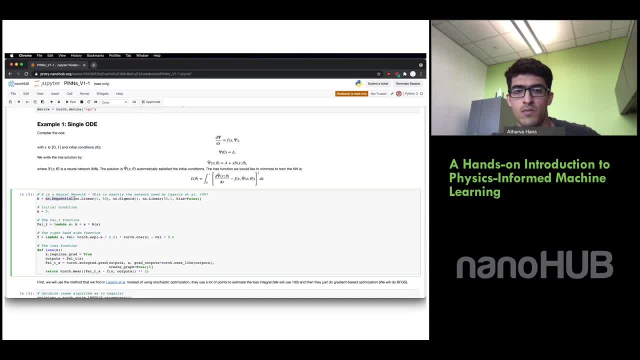 And this is basically done using the module nnsequential For this particular problem. the initial condition a is equal to 0. And psi t is our trial solution that we had chosen for this particular ordinary differential equation And, as you can see, if you plug, x equals 0,. 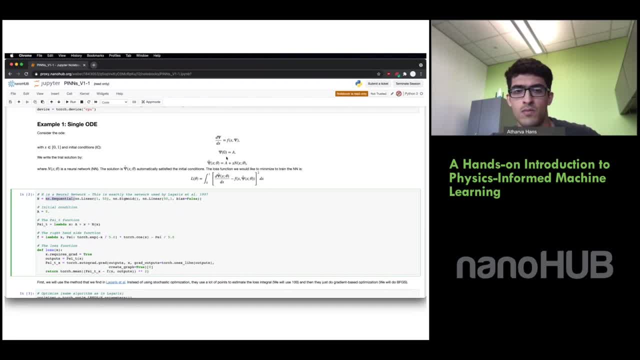 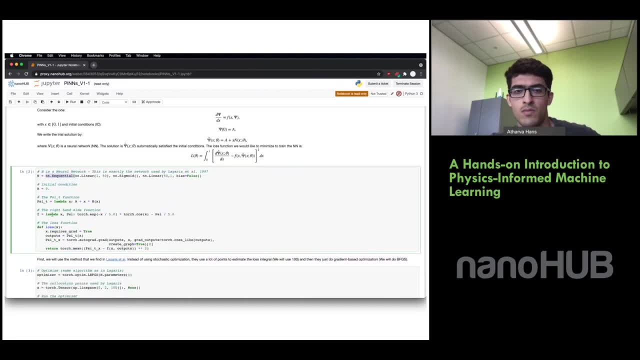 we do get psi of x equals to a, which is our initial condition. So it does satisfy our initial condition For this particular problem. the right-hand side function f of x, comma phi, is in particular this: It's some exponential negative x by 5 times some cosine minus i. 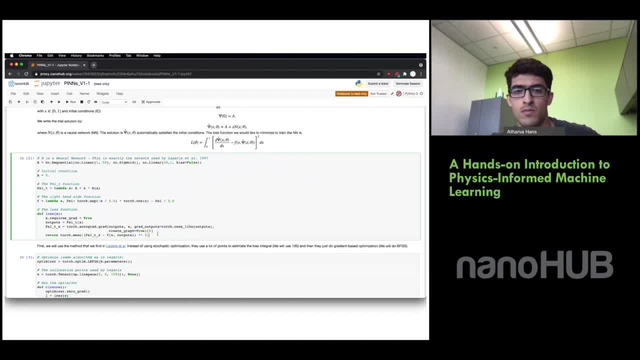 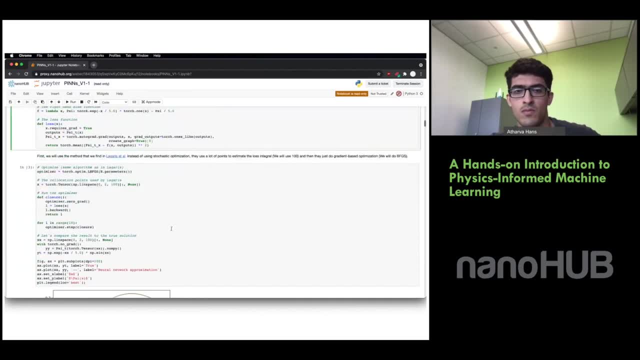 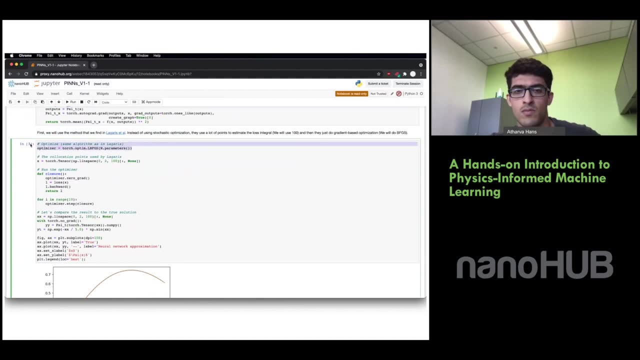 by 5.. And then I'm defining our loss function, which is this term, right here. So in this particular cell- cell number 3, we first define the optimizer that we are trying to use to solve this problem, And then we define a collection of points. 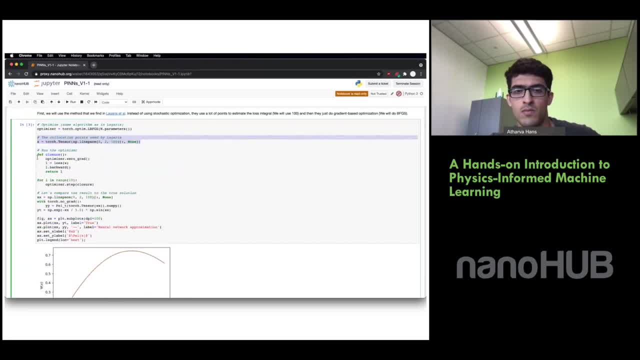 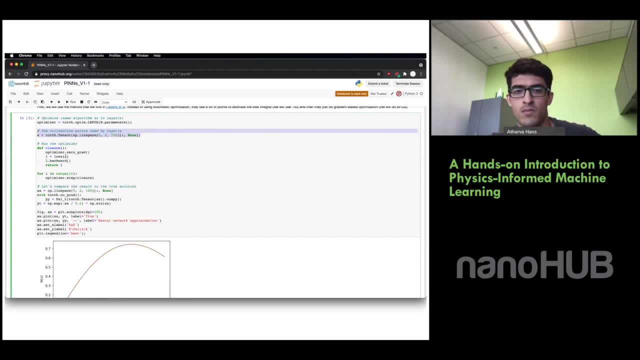 that we would like to use or which we want to solve this particular problem. Over here we are choosing a 0 to 2. And then we define a function which kind of goes over the optimization algorithm for a different number of iterations. 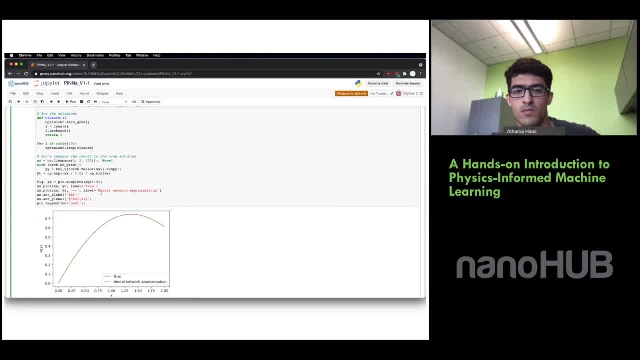 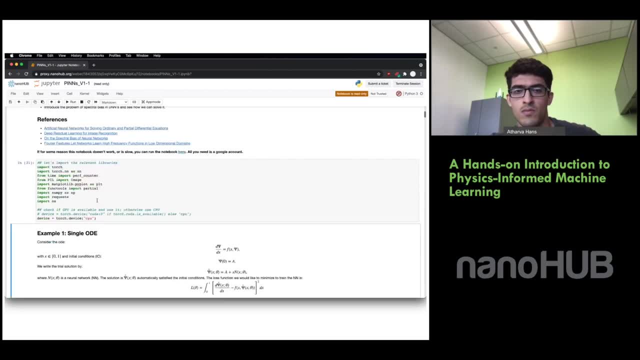 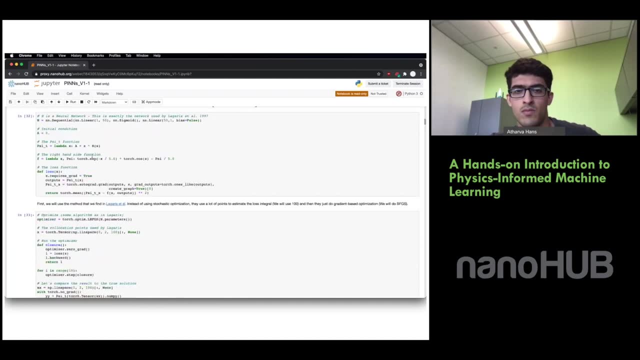 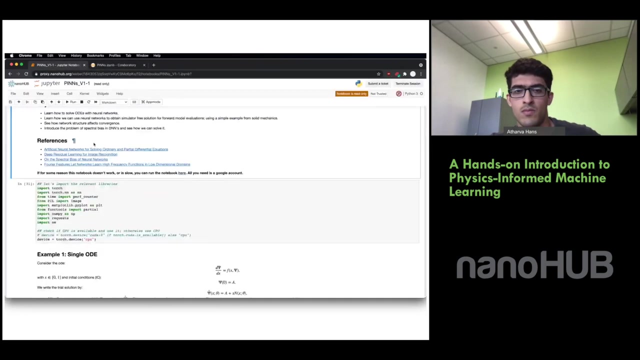 And then we essentially, if we run the cell, I need to run everything first, just a second. Yes, everyone, all participants you have to. in Jupyter, things are sequential, right? So you run the cells from the top to the bottom. 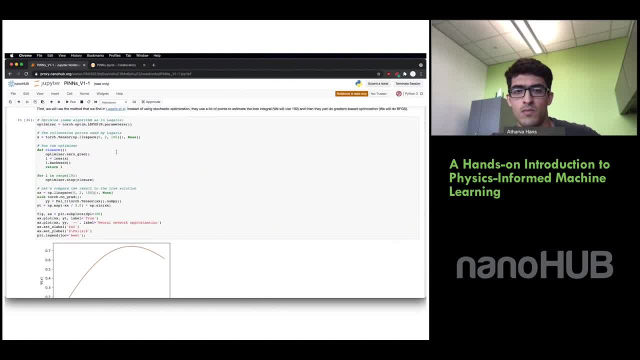 Right, Yeah, OK, so this is the kind of solution that we obtain. The blue line, as you can see, is the true solution And the dotted line is the approximation using neural networks. And in cell 4, we are solving the same problem. 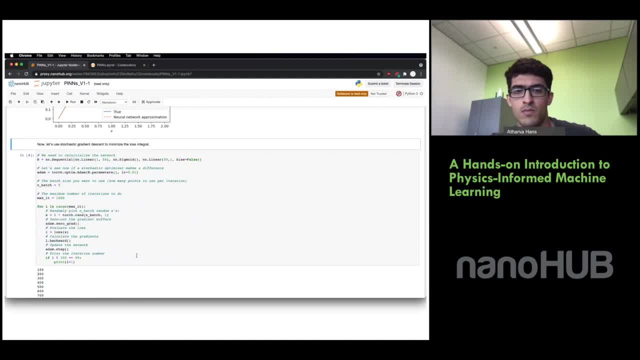 but with a different kind of algorithm, which is a stochastic gradient algorithm. So what we are doing is, instead of passing a whole bunch of, let's say, points together, we are choosing batches of points And we are trying to estimate the parameters. 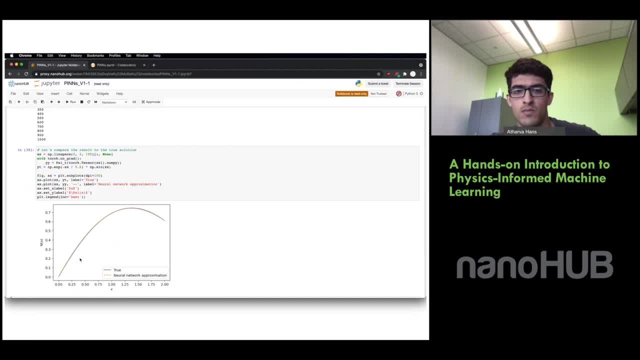 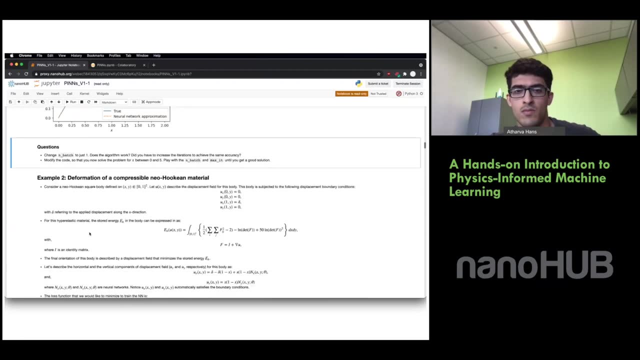 And this is the kind of the results basically look the same for both cases. So the main idea for this example was to show how we set up the loss function and parameterize the solution using the differential equation. Now I'll go to the second example. 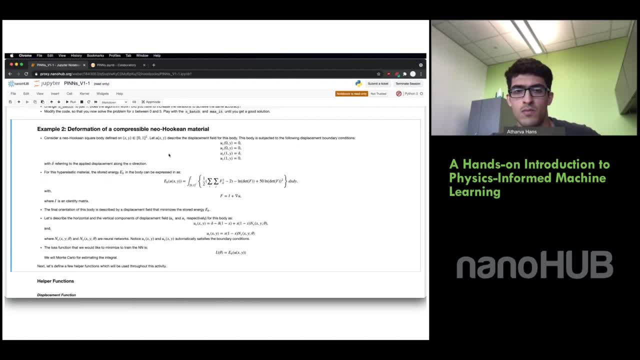 So in this example we have a square body which is defined on a one-by-one grid And the boundary conditions on this body are that the body is fixed on the left-hand side, So the displacement along x and the y equals to 0.. 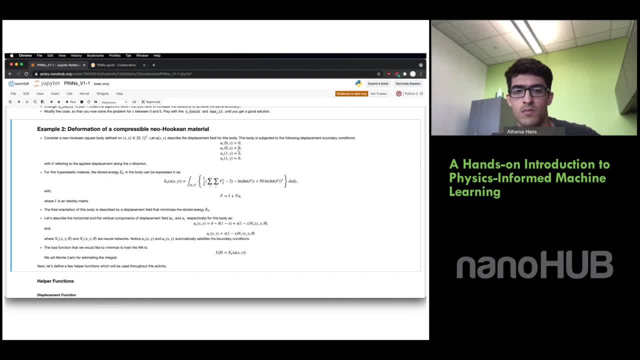 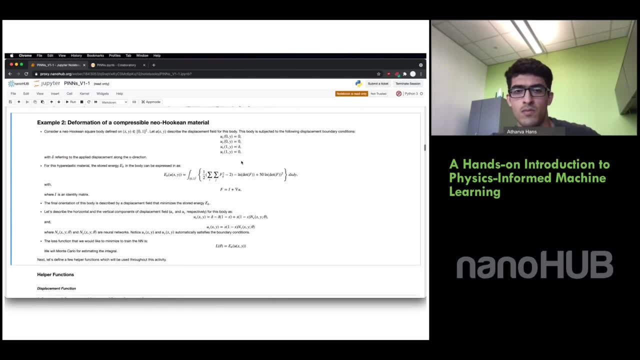 And we apply a displacement of delta on the right-hand side. So ux equals delta And uy is 0.. For this particular body, the stored energy can be expressed by this integral, which is defined in terms of the displacement field And the final orientation of this body. 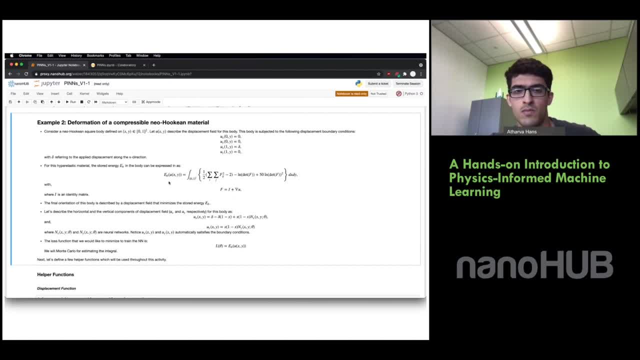 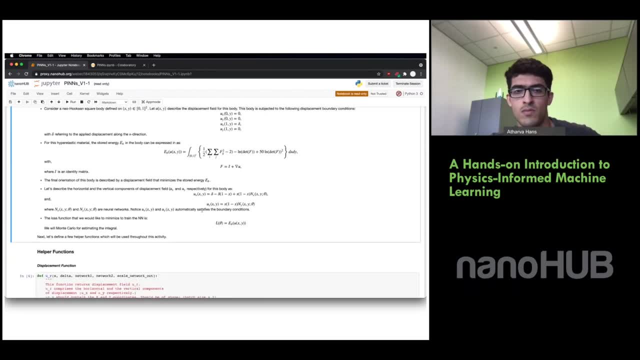 is going to be described by a displacement field which minimizes stored energy in the body. So for this particular problem, the way we parameterize the displacement field ux and uy, which are the x and the y components of the displacement field, are by using two different type. 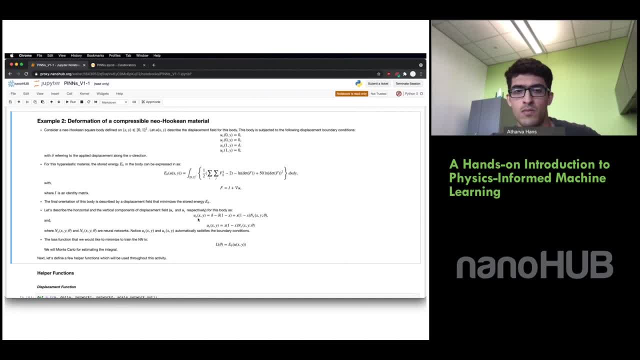 of neural networks, And this is how we do it. So if you plug, x equals to 0, we get ux equals to 0. And uy is 0 as well. So essentially, these two parameterization do satisfy our boundary conditions. 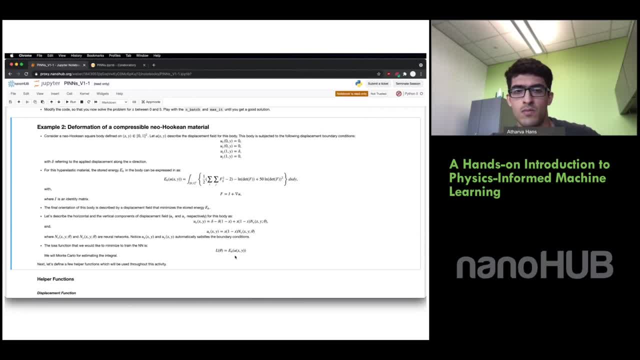 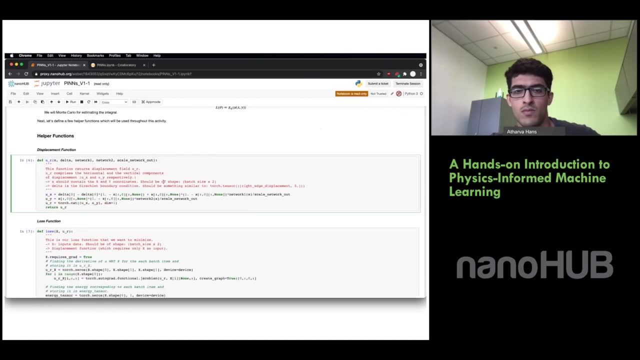 And the loss function that we are minimizing is essentially the. we are trying to minimize this energy And we are trying to find the displacement field which is minimizing this, integral. In the next few cells I am defining the displacement, the helper function which are going. 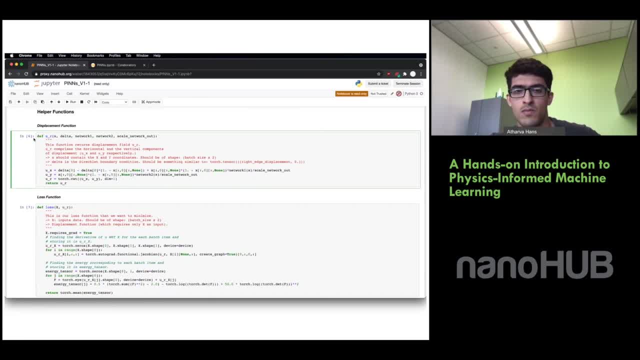 to be used for this particular example. So in cell 6, I'm first defining the displacement function, which takes as input the coordinate x, where you want to find the displacement, the displacement itself, which is delta, and the two neural networks. 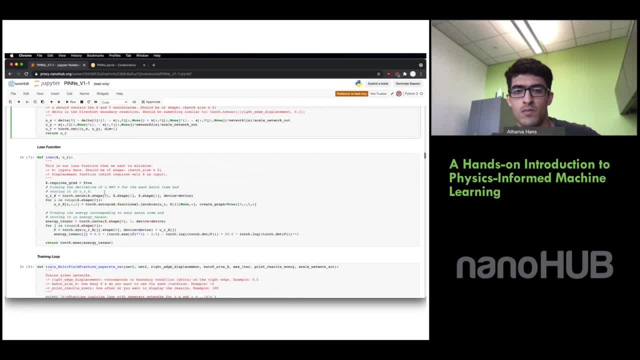 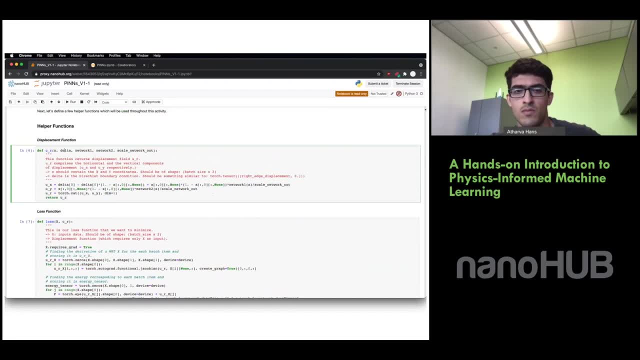 for the x and the y component of the displacement. Sorry, Atharva, can you zoom a little bit, because people have trouble on clicking. Atharva, can you zoom a little bit? I have to be here to do this actually. 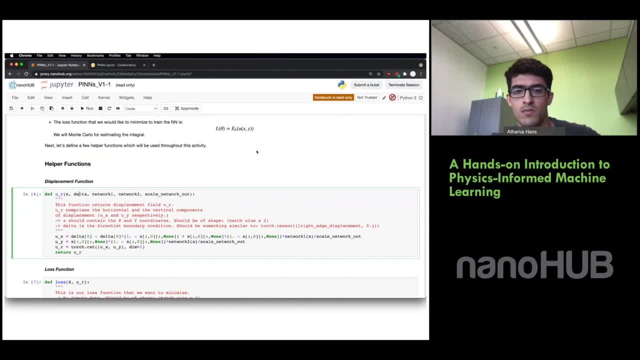 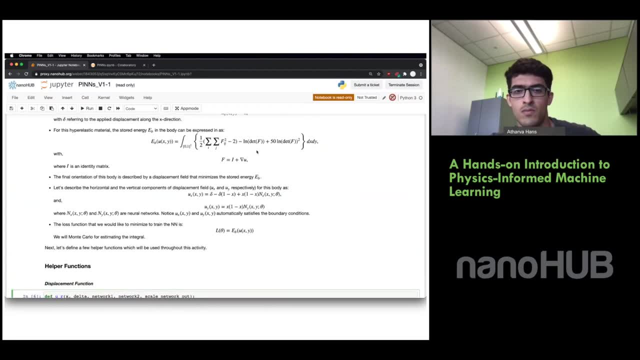 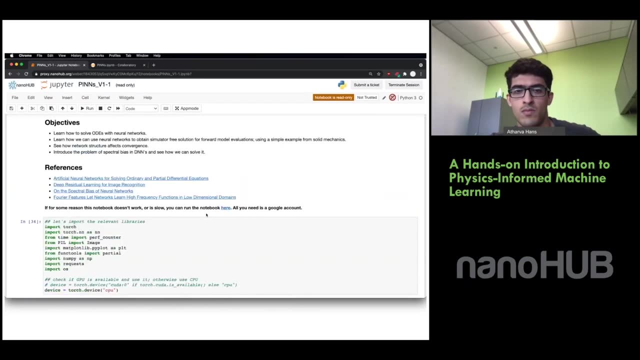 Can everyone see it now? And there's a question- Yes, there's a question- How to create our own Zupyter notebook in NanoHav, which is not uniquely lonely. So what I would say is, if people are having issues changing values- I also have a link over here. 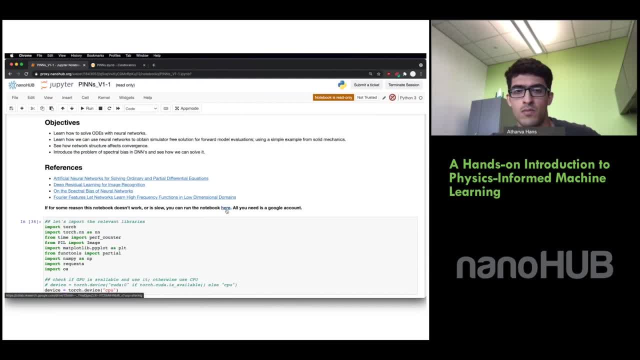 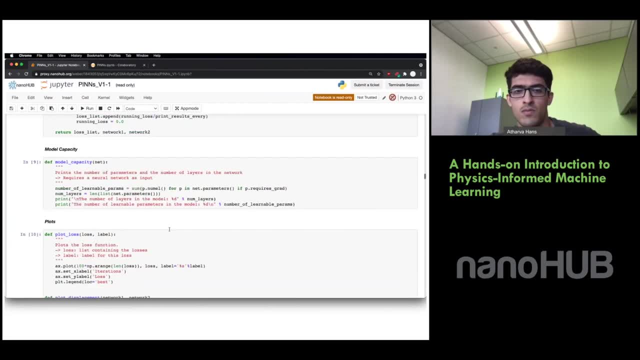 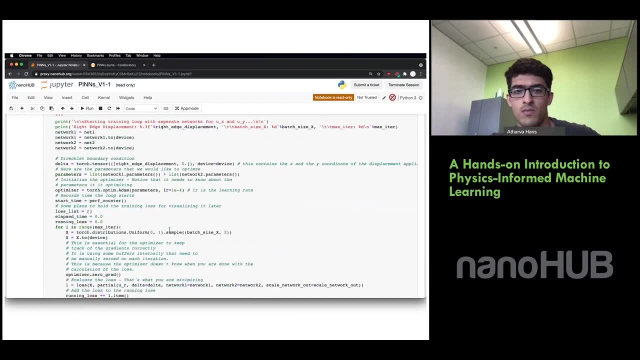 at the top of the notebook. Is there a solution within NanoHav? Yes, Yeah, yeah, let me answer this. By the way, you should be able to change whatever you want, write and run it If you want to save it. there's a couple of things you can do. 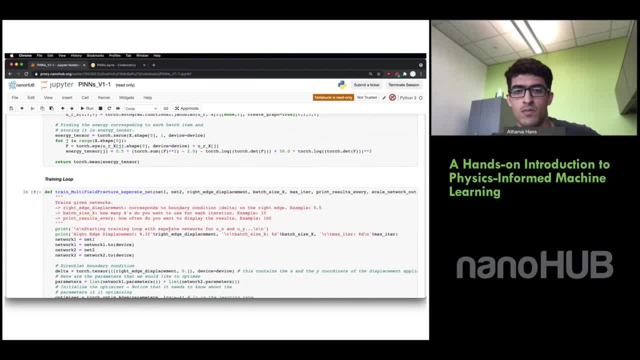 You can replicate. If you go to File, you can create your own copy of the notebook, You can download it. but you can also rename: Save As You see at the very top And when you save as it's going to be. 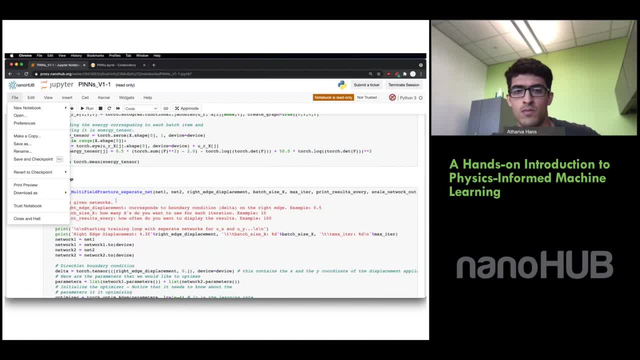 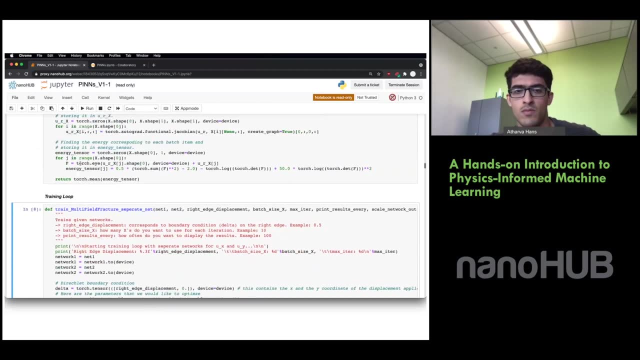 your own copy and you will be able to save it If there's a tool in NanoHav called Zupyter and you can upload any notebook directly there and run it and you have a home directory in NanoHav where you can put. 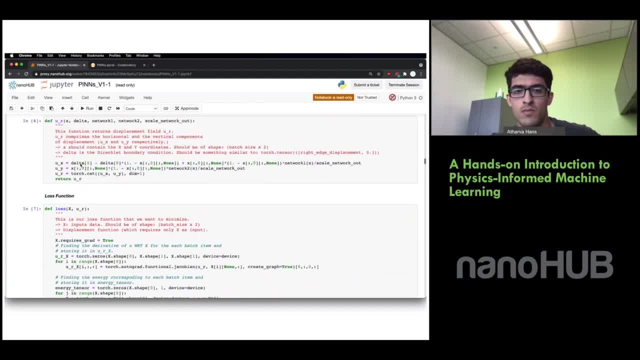 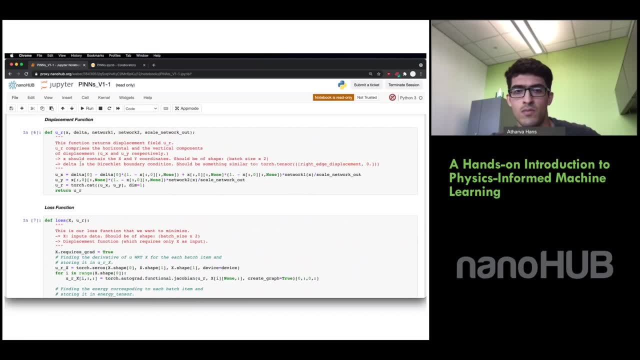 your files wherever you want. So it's true that this notebook is read-only when you run it, but it's very easy. It's very easy to make a copy of it and save it or create and move any notebook that you want in NanoHav. 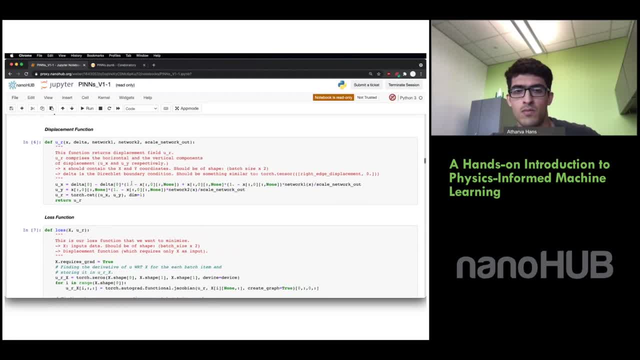 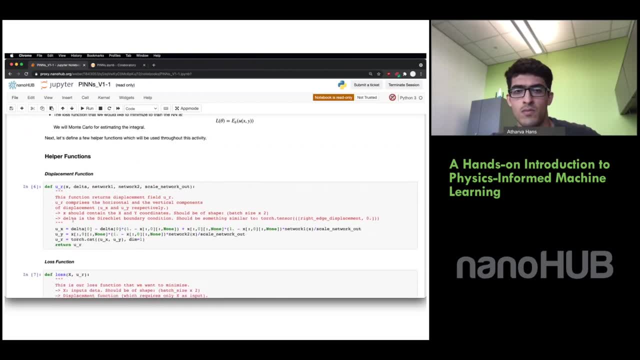 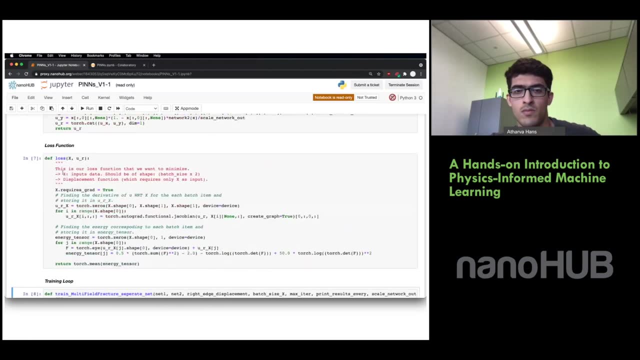 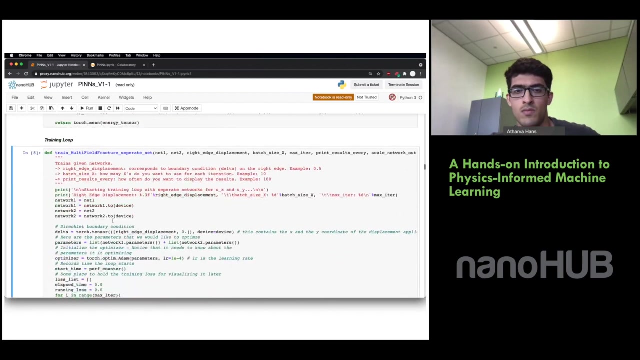 OK, can I proceed now? So here I'm defining some helper function that I use throughout the activity. UR is our displacement function, Loss is the loss function that we are trying to minimize, And this is essentially this equation, right here. And then trainMultifieldFracture is our training loop. 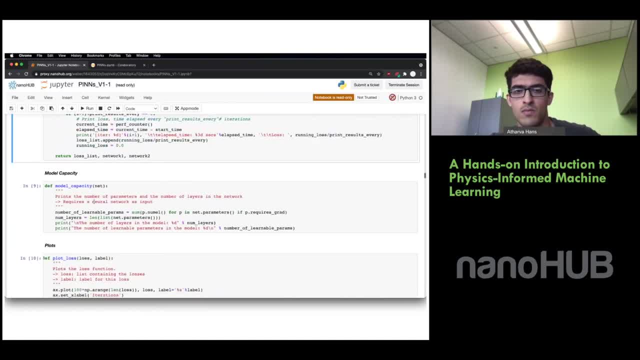 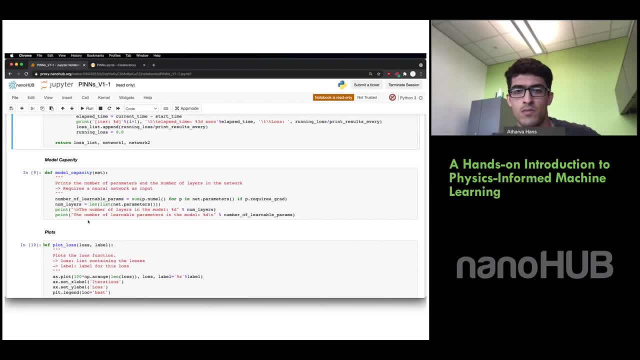 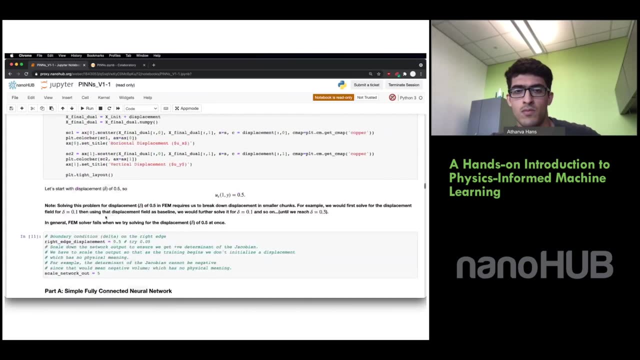 that we will use to train different networks. The function model capacity tells us the number of parameters and the number of layers that we have in our neural networks. And finally, I have some plot functions to plot the output results. So let's begin with the case where 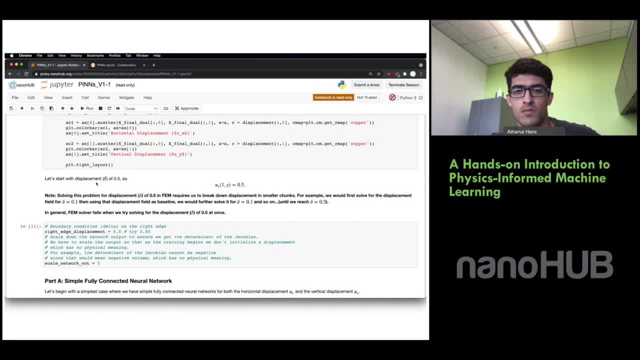 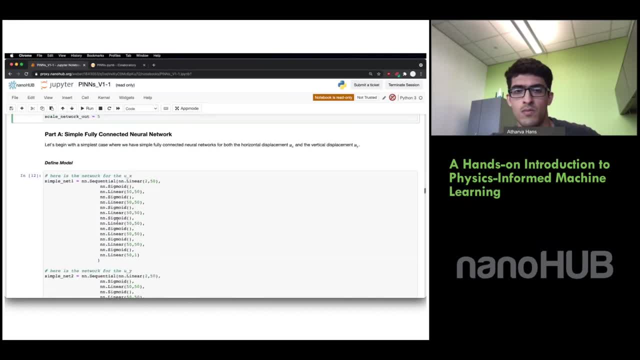 we have a displacement of 0.5. And for this particular case, we begin by a simply connected, fully connected neural network. So these are the two networks that we have And, using the model capacity, we can see the number of layers. 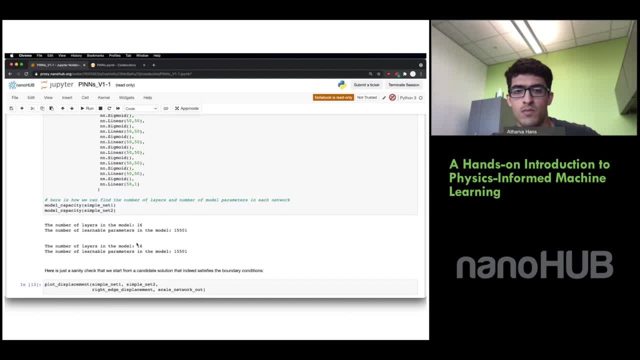 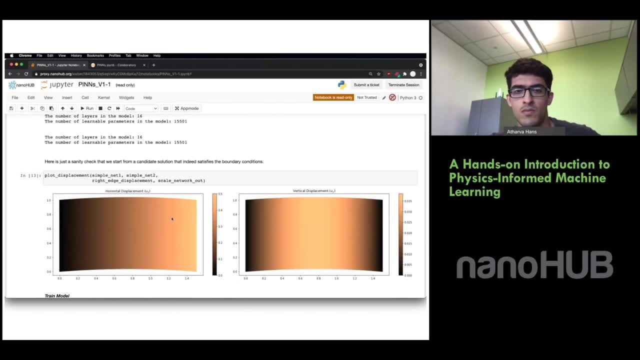 and the number of model parameters that we have in each one of these networks, And over here I'm just plotting and seeing how the results look like before training. This is to just make sure that our network kind of follows, satisfies the boundary condition. 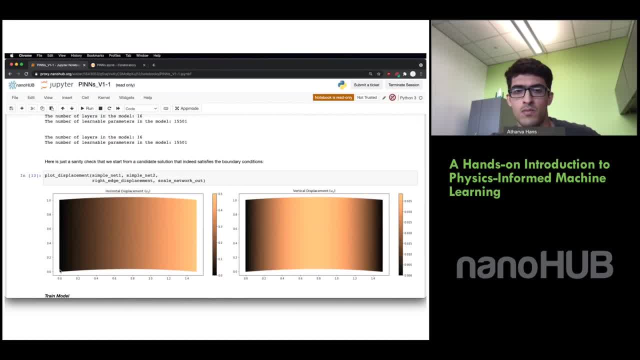 So, as you can see, ux and ui at x equals to zero- is zero And in this particular case we are applying a displacement of 0.5.. So the right edge is at 1.5.. Similarly, for the vertical displacement, ui is zero at the left and the right edges. 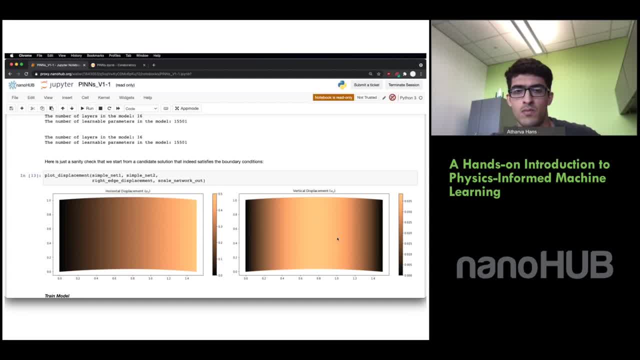 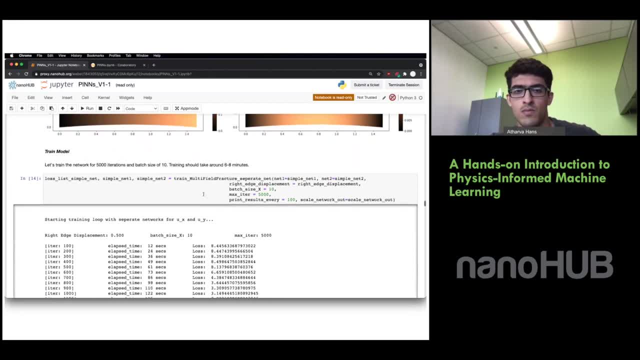 And in the center it can be anything right now because we haven't really trained the network. So in the first case, if we train the network for, let's say, 5,000 iteration and for the batch size, we use a batch size of 10.. 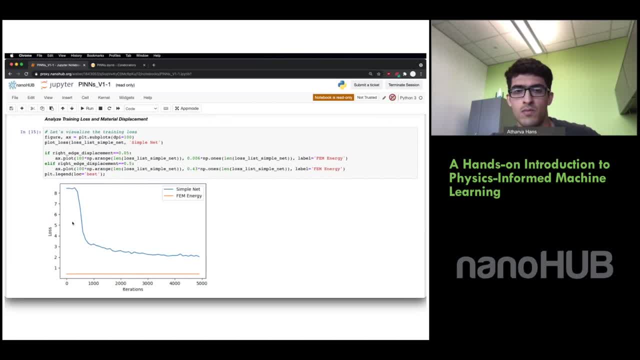 This is the kind of loss that we obtain. So here, the blue line represents how the loss is converging for 5,000 iteration in our case, And the orange line is the energy that we obtain using FEM. So, as we can see, for 5,000 iteration using a simple network. 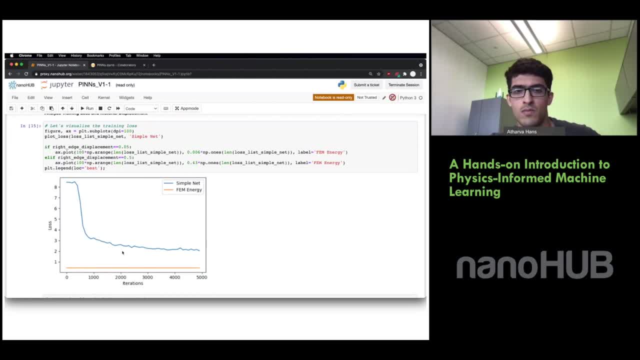 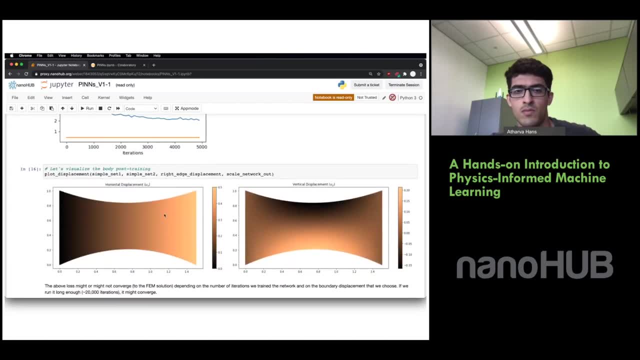 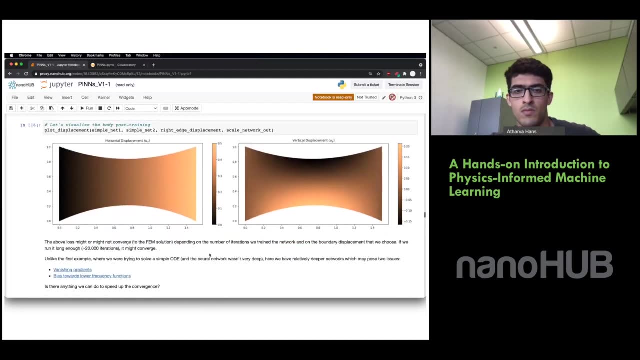 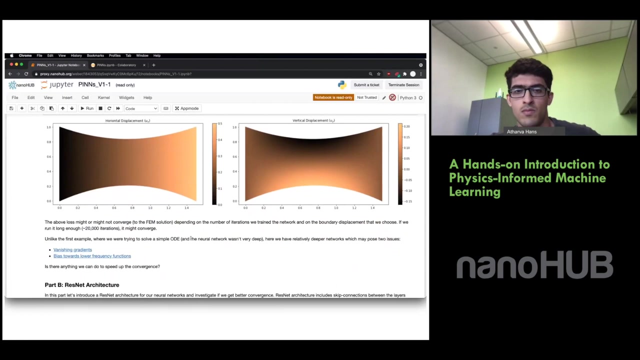 the loss doesn't really converge. It doesn't really converge to the true value of the energy, And if we use this network to visualize the results after training, this is what we get. So the issue that we might be having is, first of all, the network that we are using is kind of deeper. 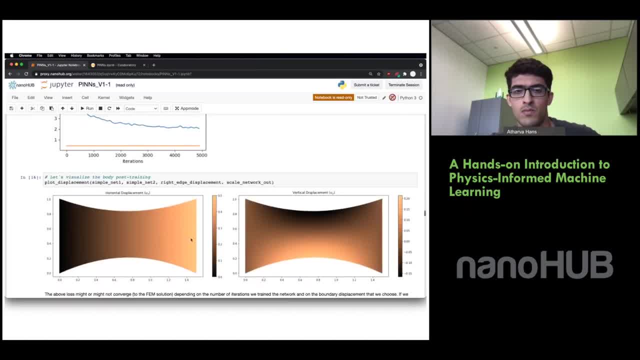 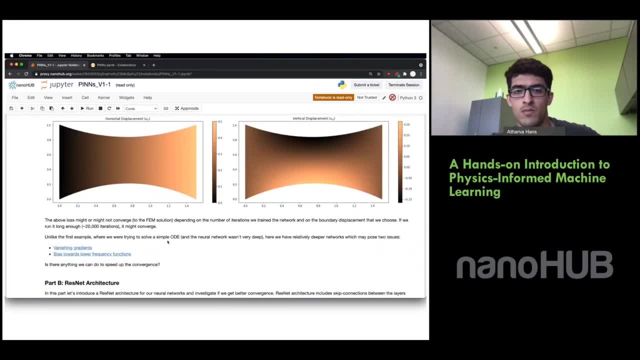 than what we used in the first example, So because of which we don't really know what we're going to get, So we might have some loss. in the first case, which we could be having- an issue of vanishing gradients, And the second issue that we could be having is the problem of spectral bias. 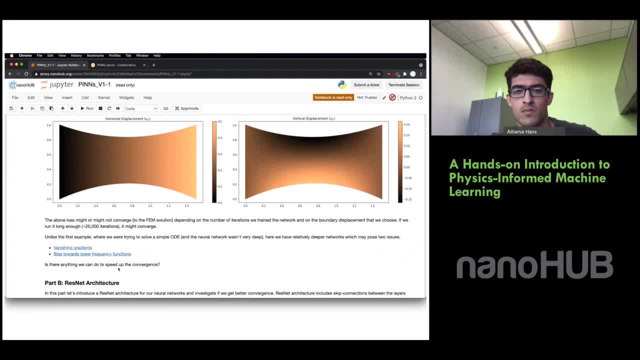 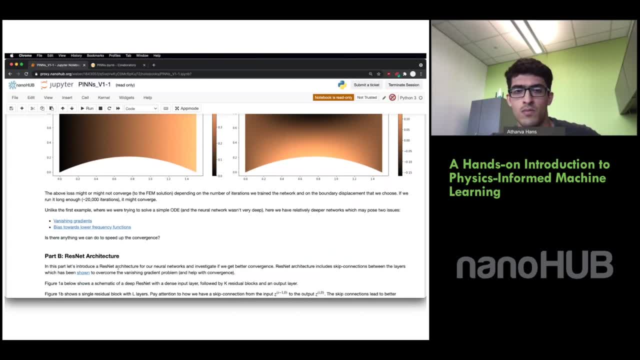 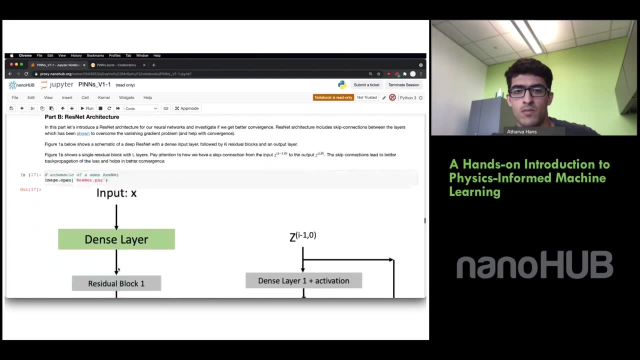 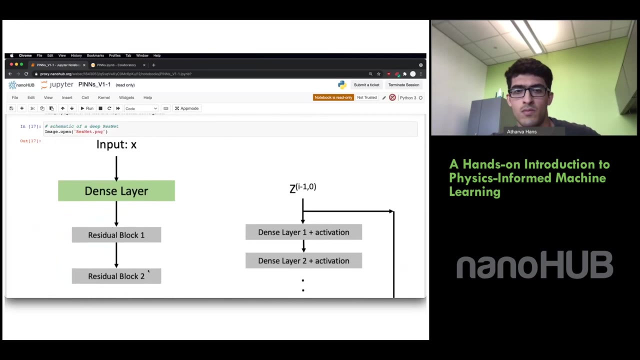 which Professor Biljanes talked about during his talk. So next we try a different type of network architecture and in particular we try residual architecture, Reset architecture. In this we have different residual values, residual blocks in the network, and the main idea is we are introducing skip connections. 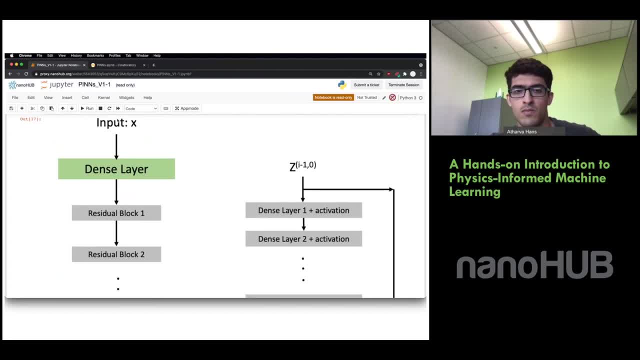 within the layers. so what happens is the input comes through the first layer and it passed, passes through this residual block, and this is a. this is what the residual block looks like on the right hand side. so as the input comes to the residual block, it not only passes through the 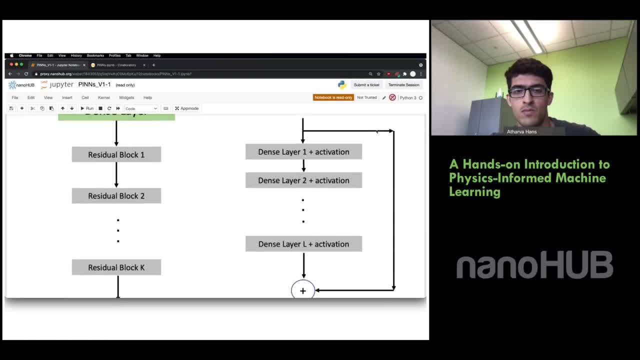 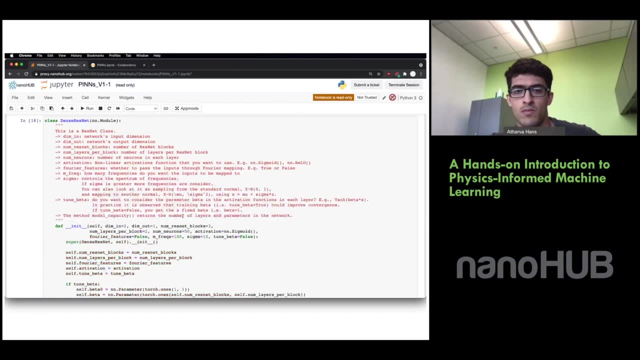 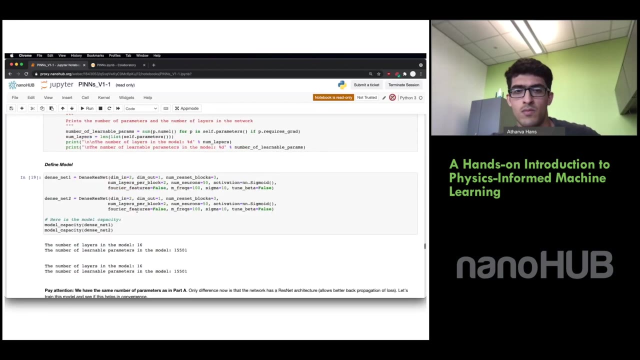 different layers inside the block, but also we have a skip connection from the input directly to the output. so that's the main idea: just introduce skip connections in the network. so over here I'm defining a resident class which we'll use to create a network, and here's a simple 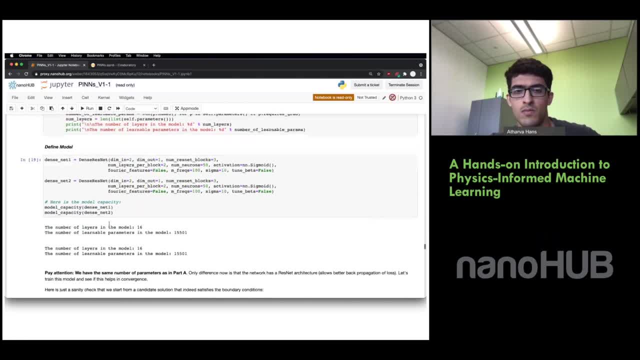 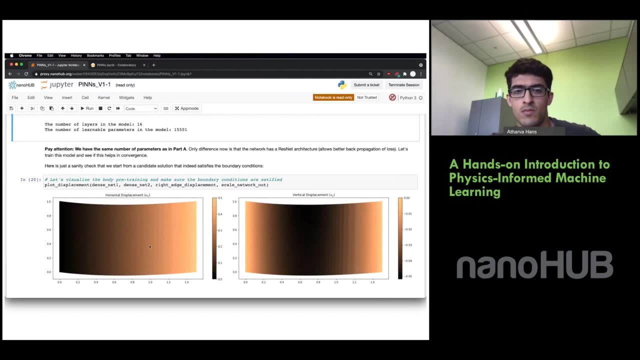 network, then step one and does not do and, as you can see, we have the same number of layers and the same number of model parameters as we did in Part A. then we had a simple, simply connected neural network and again now I'm plotting the both orientation of the body before training the network networks and once we train using this. 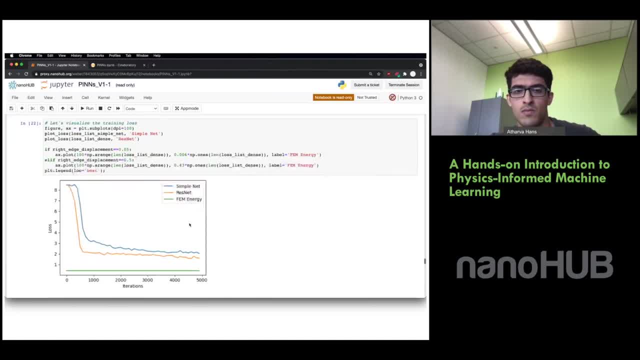 resident architecture. this is what the are loss function looks like. so, as we can see, the loss function did improve a little bit for 5,000 iterations, but we it still hasn't converged to the FVM energy. I'm sure that it's going to converge. 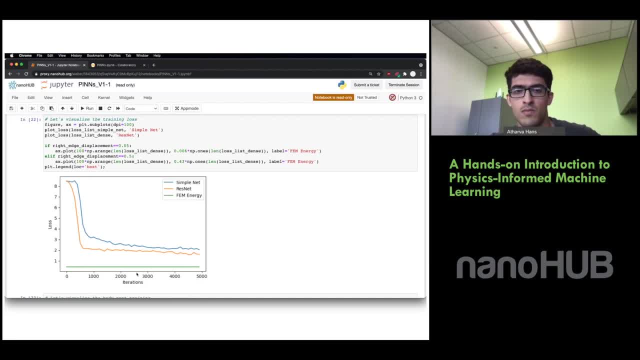 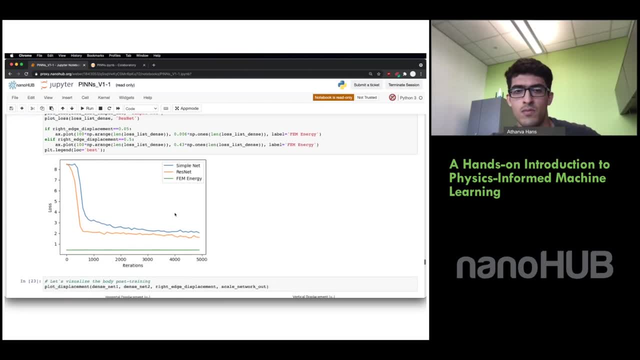 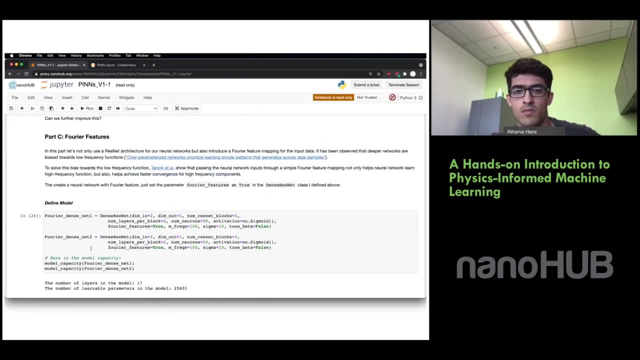 if we done it for, let's say, 20,000 iterations. but there's another way in which we can expedite this convergence process, and for that we go to part three of the example. so in this particular part we introduced a four-year feature mapping. so what? the four-year? 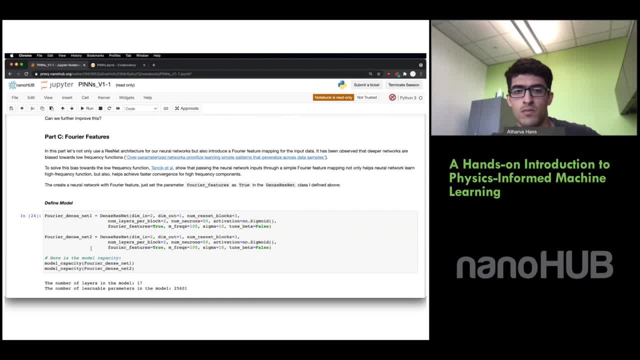 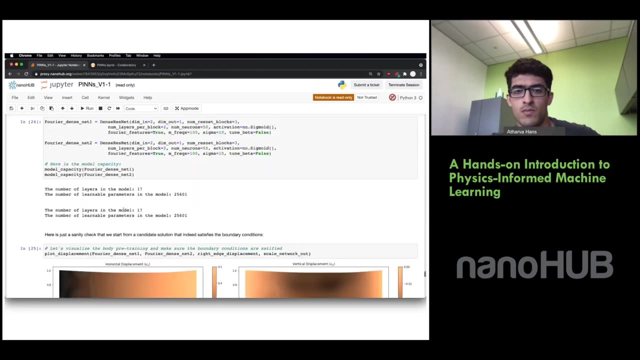 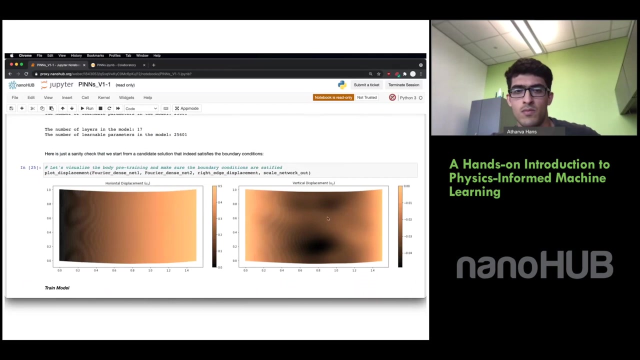 feature mapping does is it basically introduces. it basically passes the inputs through a four-year mapping and it helps the- our model learn the high frequency features in a better way. you can learn more about the read more about this in the next lecture. So this is how our the orientation of the body looks like before training and once we train this. 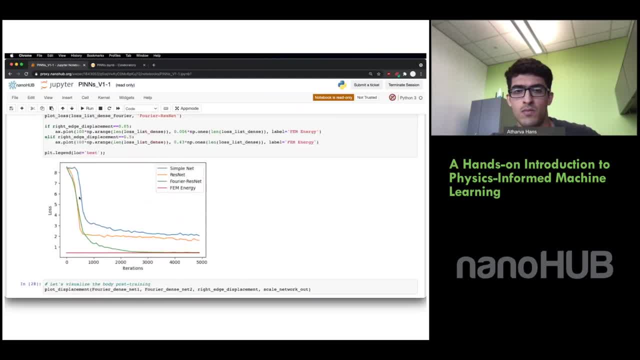 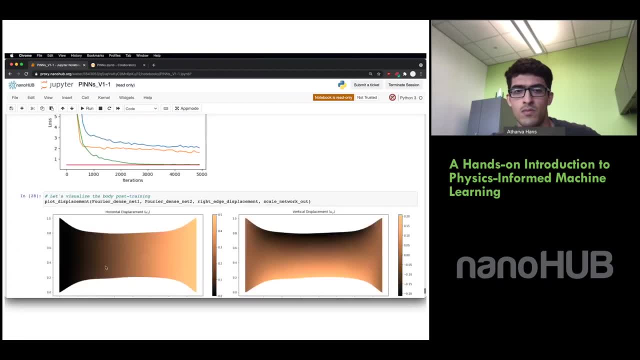 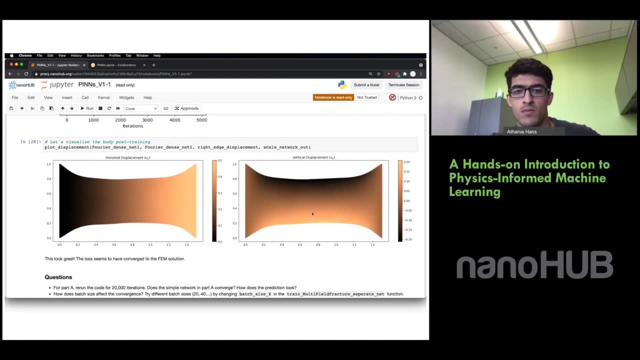 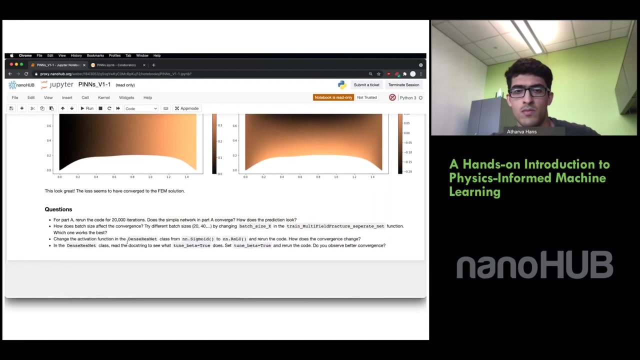 network. using the four-year feature, which is the green plot, we can see the results converge to the FVM value fairly quickly and these are the kind of results that we get. And when we compare this to the actual results that we obtain using FVM, we get pretty. the results are pretty close to the actual, the true results. so here are a few questions. when you run it, at your end you can try different things and maybe if you get better results, that's basically it. 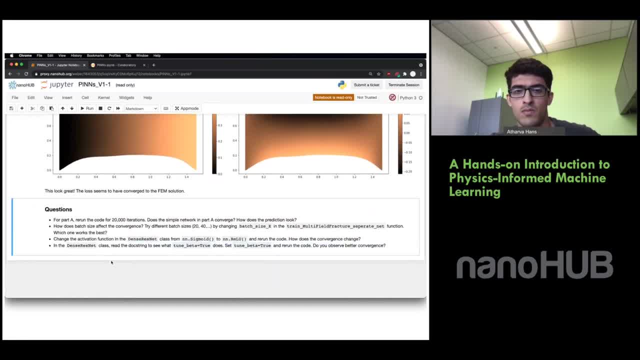 Excellent Atharva. So let me thank Atharva and Elias for a great workshop and a great presentation. very nicely done, and maybe we can take some Q&A, answer some questions outside of the Q&A. maybe, Elias, you want to take over some of the and answer some of the questions that maybe were more critical. 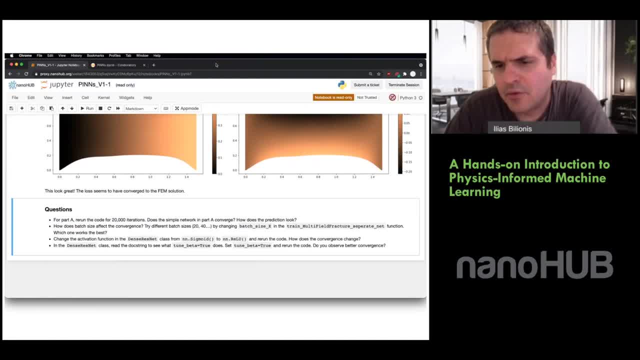 Yes. So let me see what I have answered so far. So can the energy approach we used to create a loss function for all PDEs. Is that a good question? The answer is no, You have to have an energy function, but if your problem is a physical problem and your PDE is coming from physics, it's very likely that there is an energy principle. that means, for example, straightening a equation. 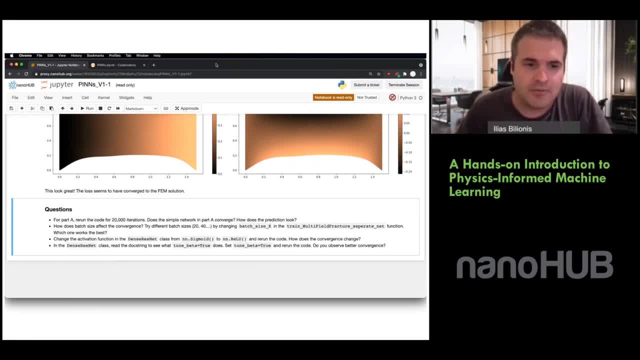 Is it possible when we have an energy function- At the end I say thank you, So it is very good. question: ground state wave function. there is an energy principle. of course the constant minimizes the energy, right? uh, if you, if you are in a time dependent setting where there is no energy, 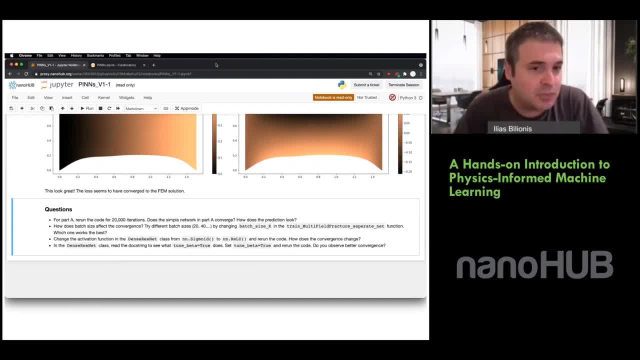 principle. there is a principle of least action or stationary action so you could use the action functional as your loss function. as far as i know, nobody has done that. there's been lots of low hanging fruit so people haven't gone with that yet. but the action is the special temporal integral of 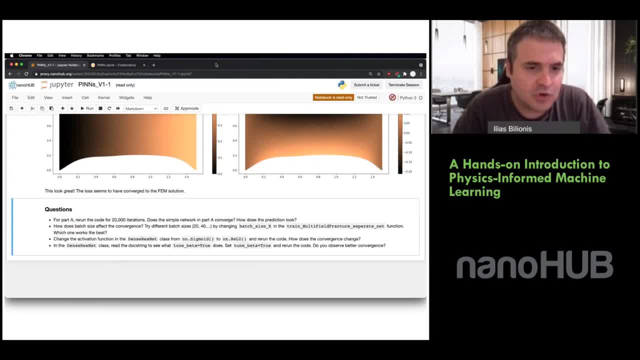 the lagrangian. so if you have the lagrangian for your system, you you can make your loss function out of that. uh, now, if you have energy dissipation in your system, if you're losing energy, then there is no action from your system that is being minimized. you're gonna have to. 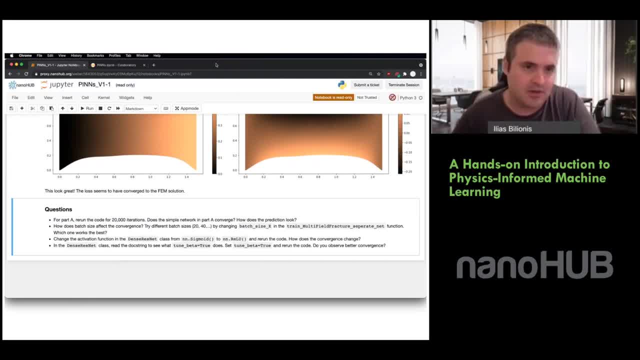 expand your system to say where your the energies go, in order to write down, uh, a principle of this action. um, let's see what other question i have here. my course is me 539, production, scientific computing, and i'm going to gradually. right now i have three lectures on neural networks. 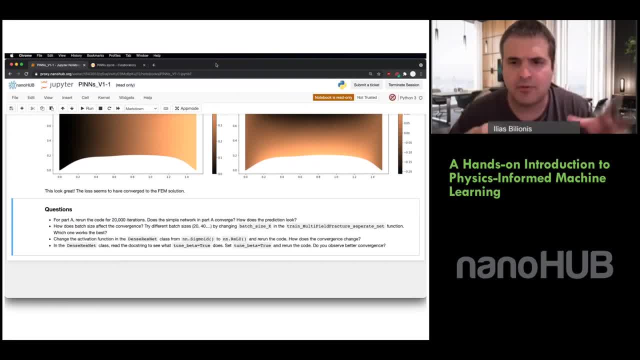 and this stuff. i'm going to make this part of the class bigger and bigger as the years pass. um, so there has been questions. yes, i was going to say one of the questions: what happens when there's multiple local optima? yeah, you are screwed, that's what. 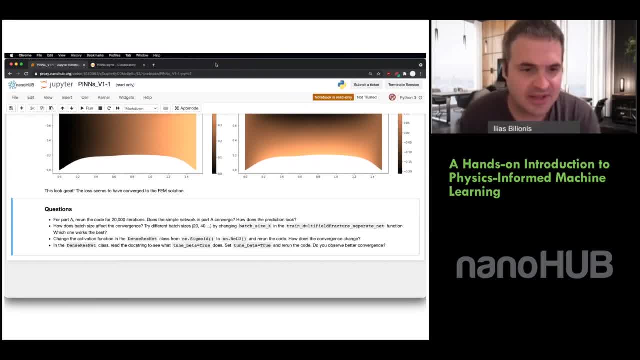 that's what i'm saying. if you try to use this lively in your problem- because we're still at the beginning, as we understand everything, uh, how to use this technique- you're gonna get into one of them. okay. now, if you're doing stochastic gradient descent, there are some theorems that show that. 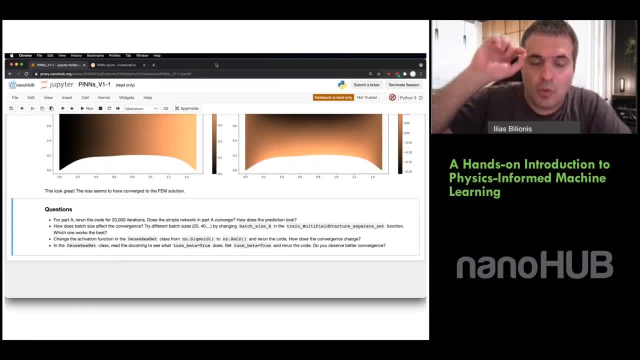 stochastic gradient descent will actually jump over bad local okay. so that's why you should always use have some stochasticity way you minimize the problem. If you want to learn more about that, you should go and read Michael Jordan's Stanford professor on this topic, on the convergence of stochastic gradient descent. 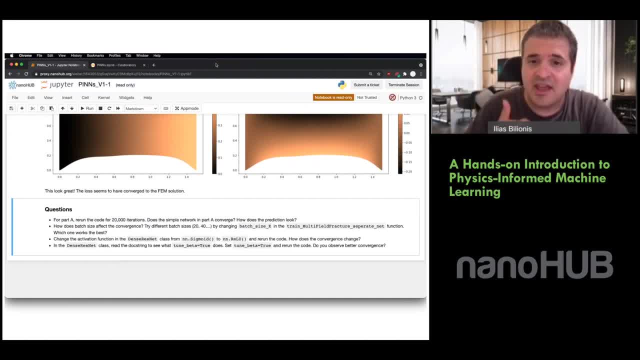 The other thing is that if you have an energy principle, then it is very likely that you have a single minimum. That's why you should use the energy function if you have it. Other question: I want to mention a little bit about data right. 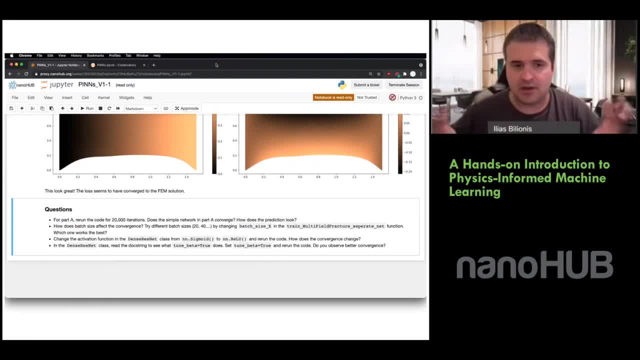 So what we did in this hands-on activity has no data. We just directly use the physics to solve the PDE or the ODE, and you could extend this to solving the ODE or the PDE For many different parameters in one sheet, for all parameters in one sheet. 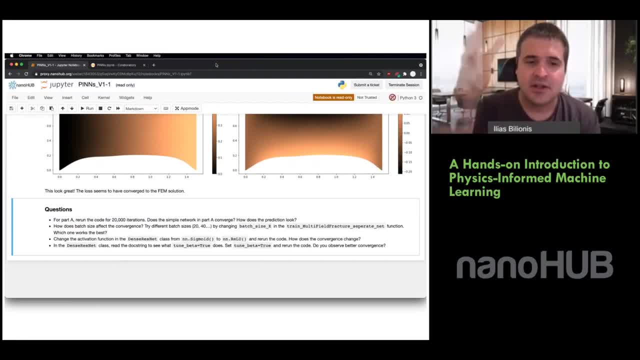 Now, if you have data- so let's say that you have a Tharva's problem in the neohokian material and you also have some strain measurements- okay, You could use this data to augment your. so you could essentially use both the data and 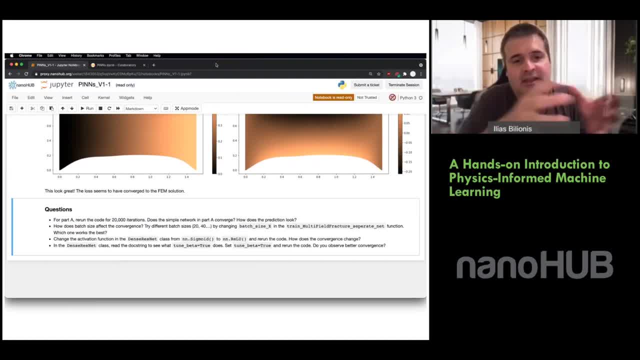 the physics. How do you do that? Well, you have a data part for the loss function which is basically the sum of square errors, sum of the squares of the errors of your predictions. That's one part of the loss function. and then to add to that, you add the physics-based 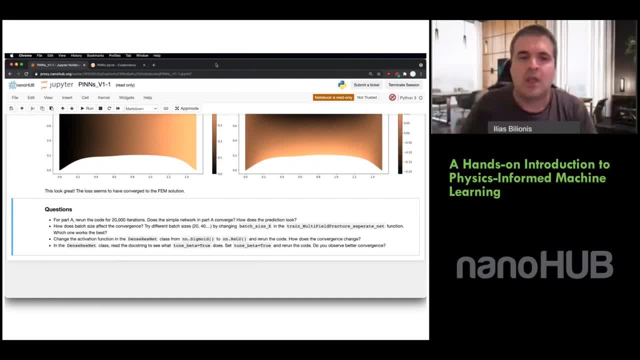 loss function. So you combine the two and then you minimize that and then you get basically the ability to extrapolate beyond the data, Beyond the limited data you have, to the entire domain, because you're using the physics to pass any holes you may have. 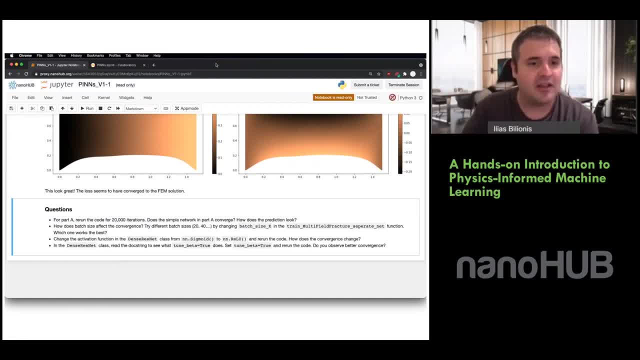 And then if in your physics you have missing parameters, you can also add these in your optimization problem and then have a nice data assimilation calibration problem. Maybe one more question, Elias? Yes, Before we run out of time, Yes, 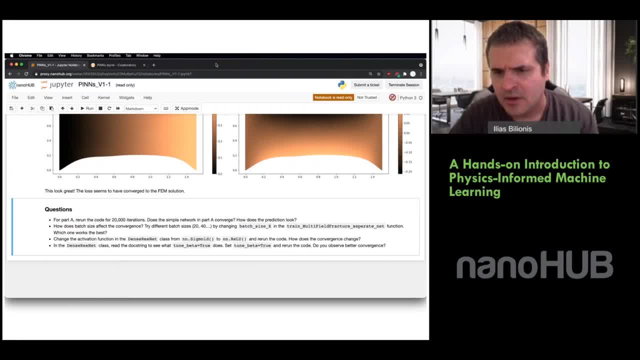 I'm trying to get to the end where you have data but you either don't know that physics or have an approximate knowledge of it. You have touched the basic research question that is on the mind of about everyone right now. So the idea would be to parameterize the physics somehow. 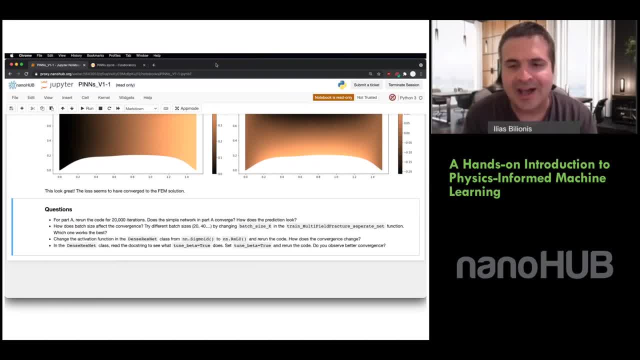 So, for example, one idea would be to say: I don't know the right-hand side of my equation. I'm going to make it a neural network and I'm going to try to fit it as well. So you have data, you know that there should be some differential equation. you don't know. 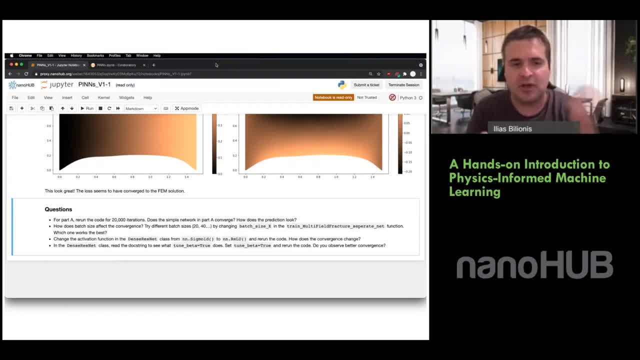 exactly its form. you parameterize it and you create now a loss function that has the physics with a parameterized OB and data and minimize that. Hopefully that will recover the physics. There is a- It's a very hot topic- how do you learn physics? 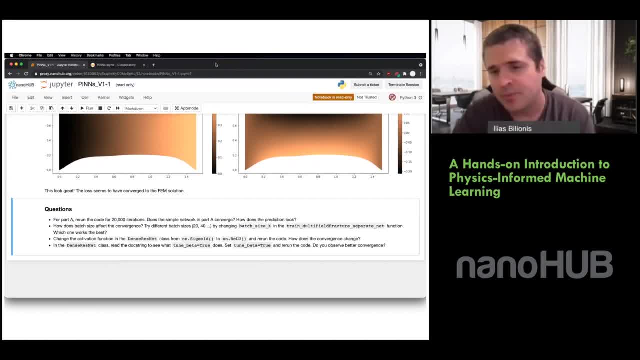 You can say: I'm going to learn the Lagrangian, for example. Again, not all physics. Again, no one has done that to a satisfactory degree so I cannot give you any references. but if you go to conferences on statistical classification or computational science in, 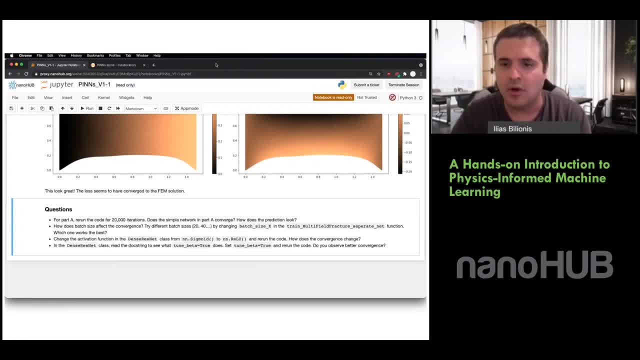 engineering. there will be at least two attribution portions on just that. How can we extend this to density functional theory? You could, in principle, use this to, So you will have to go to the energy principle Right, You could use the minimization. 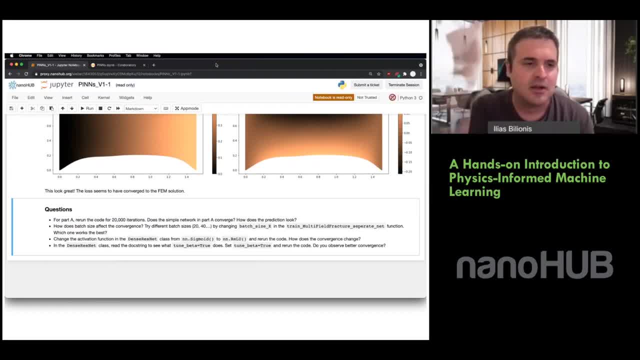 If you can pose the problem of finding energy density as a minimization problem, in principle you could use this technique. It will work better than density functional theory. Has somebody done it, If it's not already done, because there are about 200 papers per week on the topic, somebody 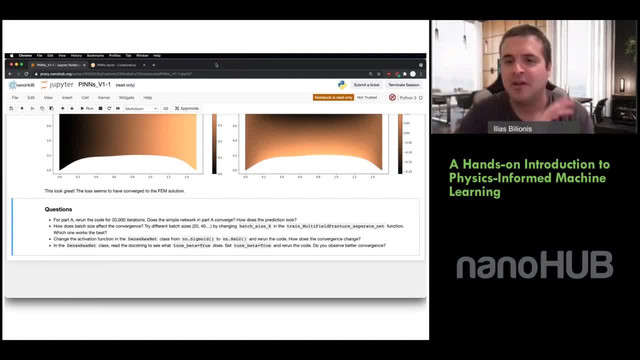 will do it, try it. I don't know if it's going to work, Maybe in the next few months, I don't know. I don't know, Maybe in the next few months. How do you measure physics? Same question as before. open problem. 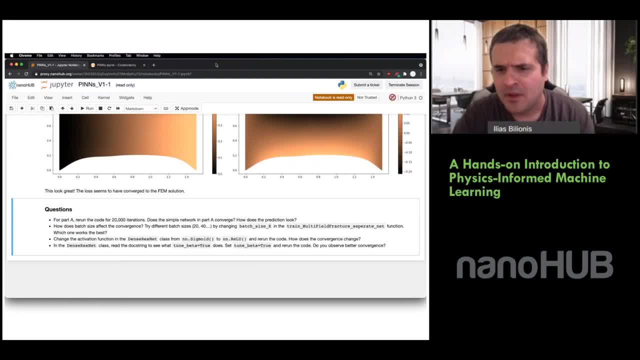 What did you have data on? I think I covered all the questions. for audience, Would L1 loss Post slides- Google post slides L1 loss function? should the network ignore noisy or chaotic features in the physical models? Good point, I did not know. 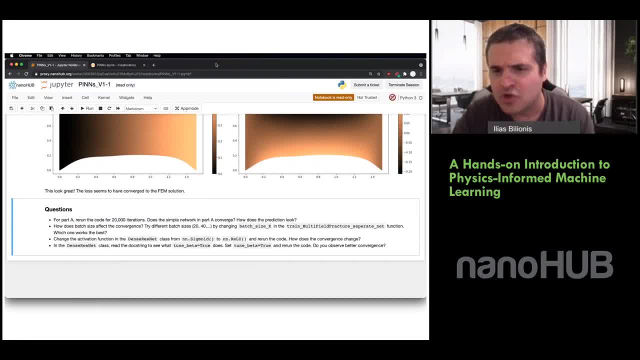 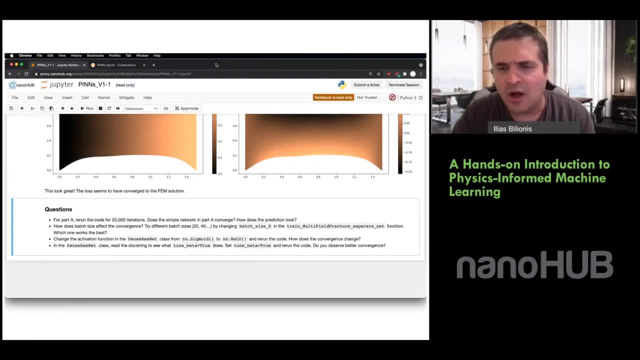 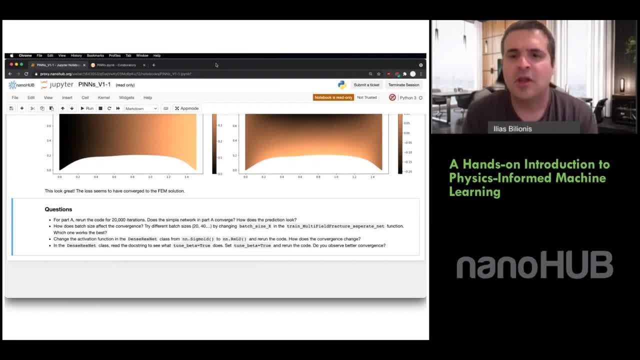 the MSC loss? Very good question. Here's the advantage: You don't need a solver for your physical problem. Okay, That's one advantage. And in high dimensional parameter spaces, the problem of generating training data and minimizing the MSC loss doesn't scale. 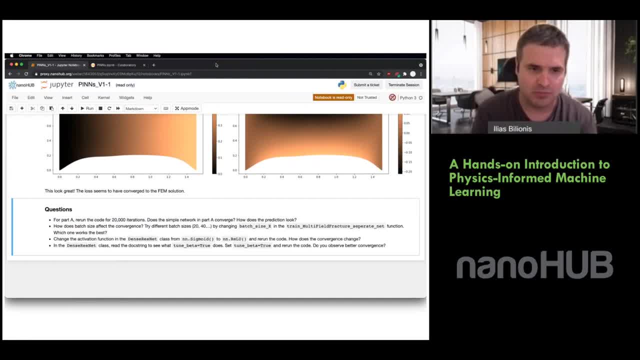 We need so much data. We need so much data. That's impossible. There's a curse of dimensionality. It is written that Monte Carlo is used for the integral. What does this actually mean? Does this have any significance to the final accuracy?